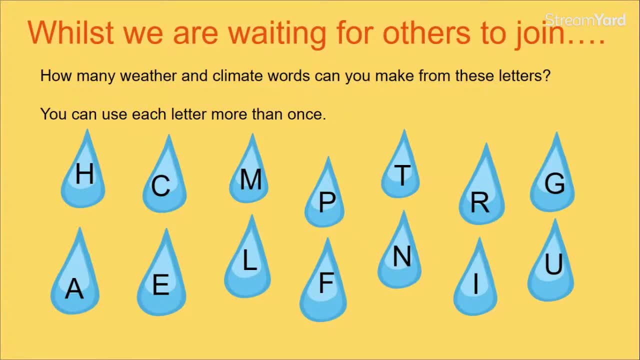 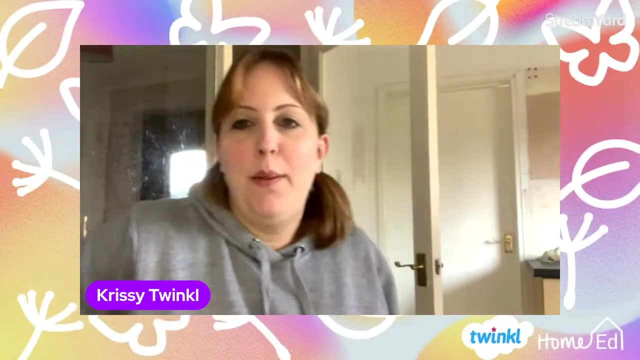 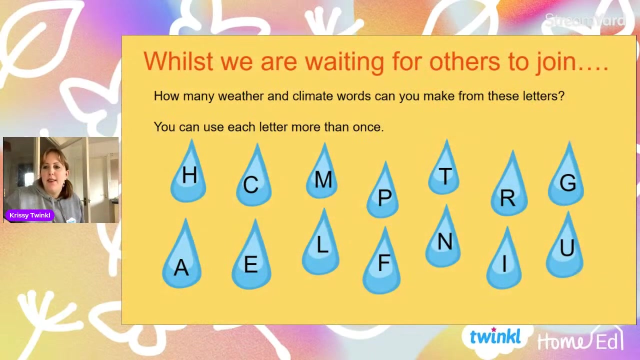 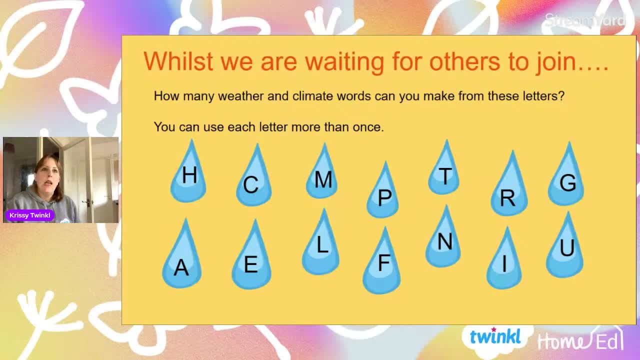 And last week I gave you a really key geographer's skill, which is how to draw a climate graph, And I talked through to you, even if you go all the way up to GCSE and you're asked: what does this climate graph show? All the things that you need to include when you're writing about climate graphs. 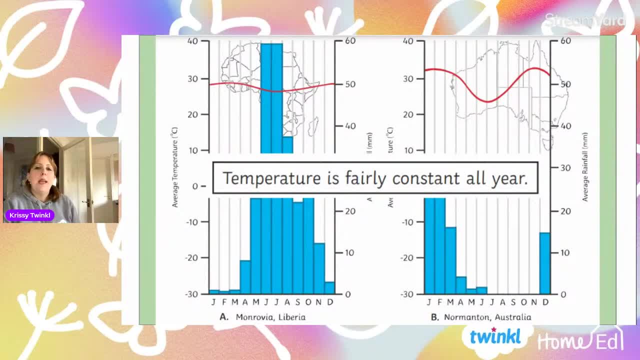 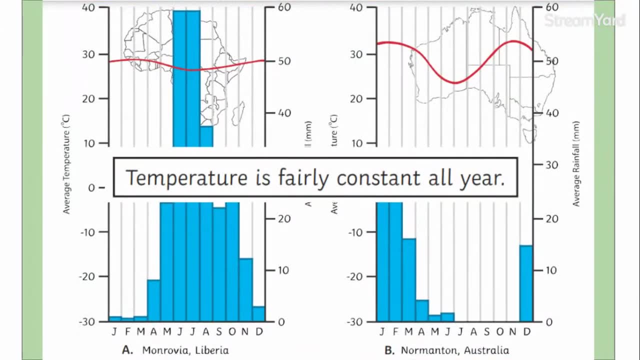 Now, today, what we are going to be looking at is: we're going to be carrying on with this and we're going to be looking at climate zones. Now I'm going to turn my camera off so you can see this, But these are two climate graphs, a bit like what we were looking at last week. 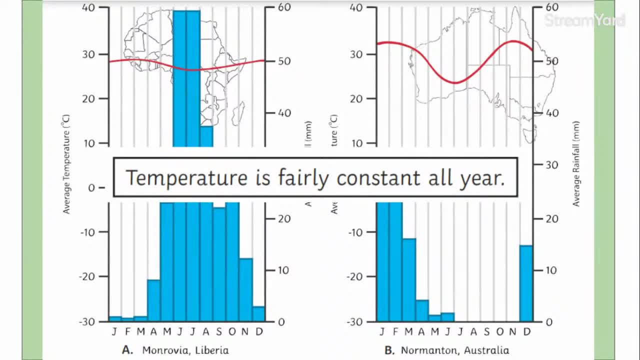 Now, which climate graph suggests that temperature is fairly constant all year? So what can you remember from last week? So we have Liberia and we have Australia. Which of these climate graphs show you that the temperature is roughly the same every year? So if you want, we'll call the one on the left, number one. 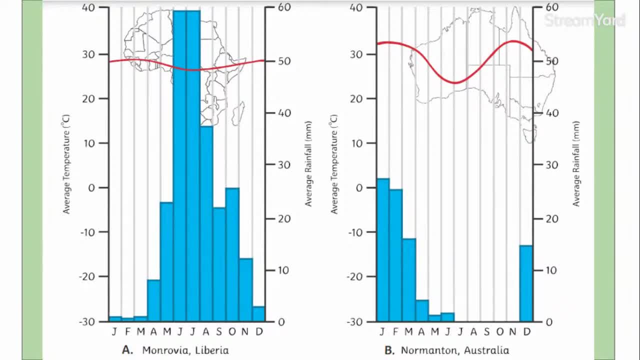 And the one on the Right, number two, or we can go for the one on the left is A and the one on the right is B, to save you sharing Liberia or Australia. But which one is it that has the temperature? Now, if you remember that the temperature is shown by the red line graph and on this one, remember I told you always have to look at the axis, because sometimes the temperature is shown on the left. 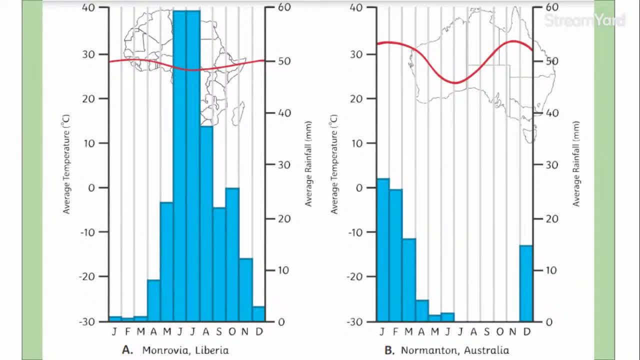 And sometimes the temperature is shown on the right. So you have to look carefully. So you should be on this one, The temperatures being shown on the left, And it's shown by the red line graph, And so you should have A. So the constant temperature is a, because if you look at that line graph on A, it's roughly 28 to 29 degrees all year. 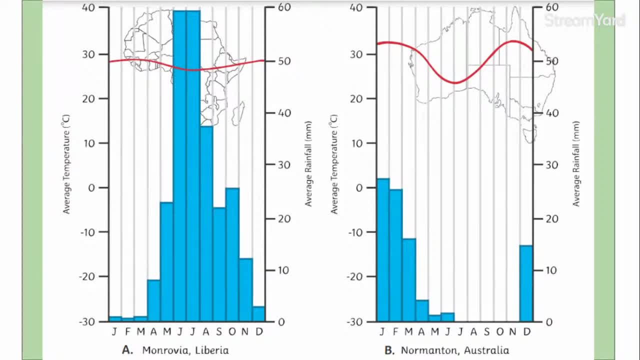 And when you get to one of those differences, you're right to a complete difference. And the temperature and the temperature is shown by a red line graph And sometimes, with temperature, the temperature is shown on the left, Sometimes the temperature is shown on the right. 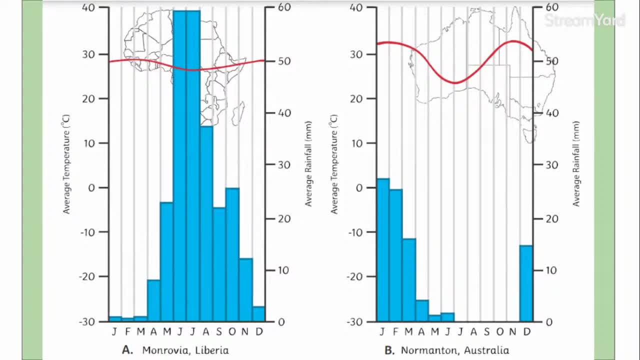 So you have to look carefully. So you should be on this one all year. but if you look at australia, can you see? some points of the year it's about 32 degrees and other times of the year it's about 22 degrees. so there's a 10 degree difference. so well done. 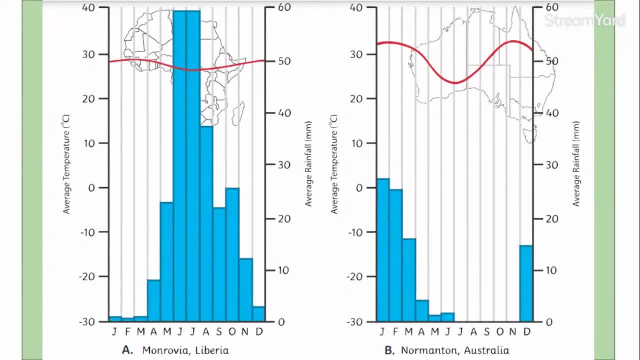 if you've got a or one, or liberia, because that is the one that has the fairly constant temperature, right the next one, which has a dry season from july to november. so you're going to be looking now at a place that doesn't have any rainfall because it has a dry season. so you 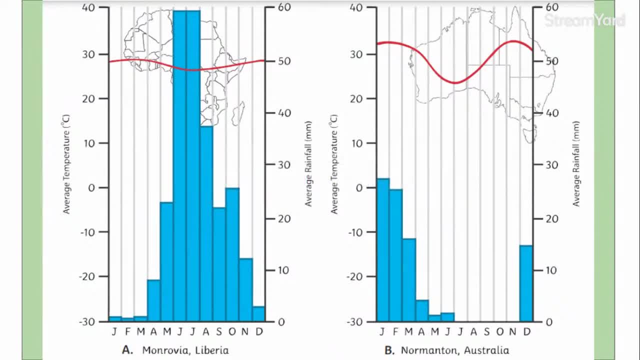 should be, therefore, looking at the rainfall, and rainfalls are shown as bar graphs. if you remember, we have our bar graphs and blue bars. so which has the dry season? is it a or one or liberia, or is it australia or b or two? well, we're far, far, far more uniform on this. i think our brains are starting to remember now. 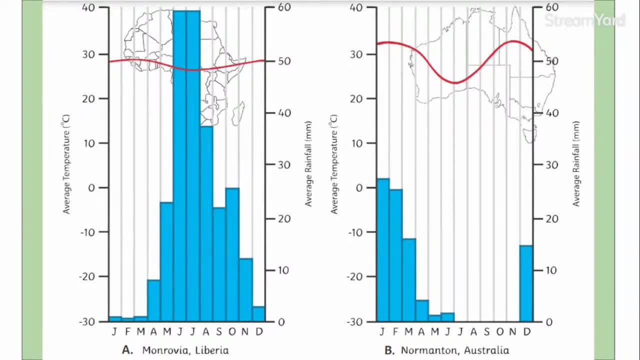 that it's climate graphs, because absolutely b is the correct answer. so australia has this dry season from july to november, because you can see there's no bars at all, which means there's no rainfalls. so which has the dry season? is a or one or liberia? or is it australia or b or two? 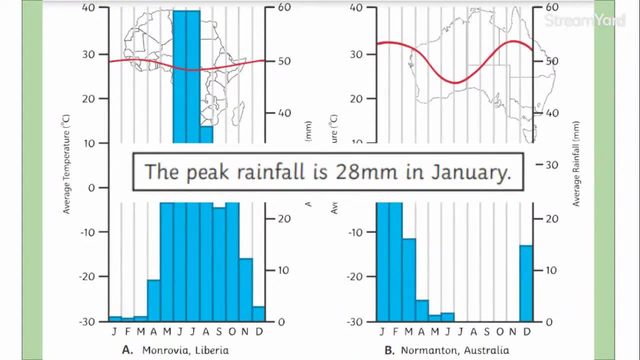 rain Right, which place has a peak rainfall of 28 millimetres in January? So now you're looking at the right axis, the axis on the right, So which has, in January, 28 millimetres? That's the peak rainfall. What are we looking at? The peak rainfall. You're right, it is B. Now do you know? 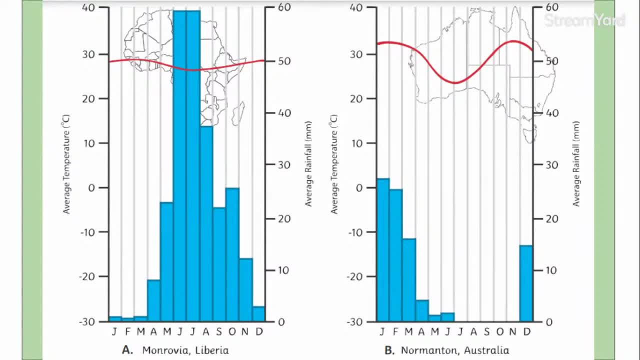 what I started doing. I started looking at the temperature going. oh, I can't remember what the answer is now. I did that age-old mistake of looking at the wrong axis. But lots of you are definitely going for B, because you should be like scooching that bar across and it's roughly on 28.. 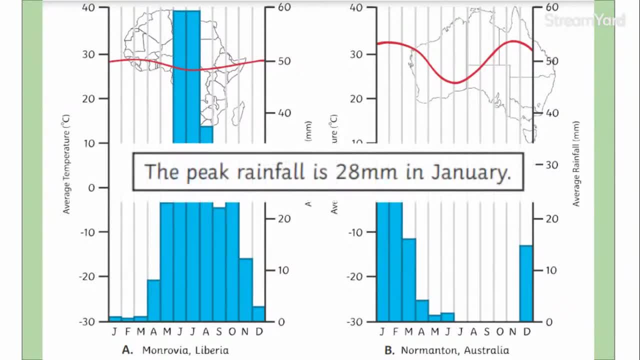 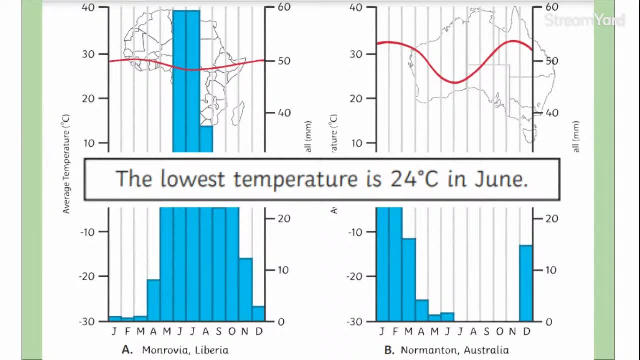 See, even I sometimes get a bit confused. that's why I went quiet. I was like the camera. I don't remember what I'm looking at now. Right, the temperature. so we're now back to looking at the line graph. The lowest temperature is 24 degrees in June. So which has the temperature? 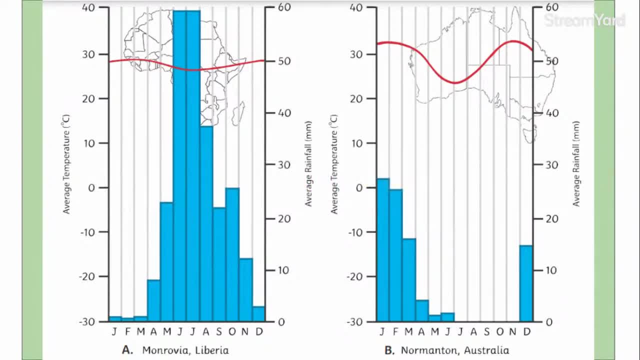 of 24 degrees in June. So looking at the bar, not the bar, the line, I'm confusing you. I need to be quiet. Looking at the line which one's 24 degrees, Absolutely it is B. So it's quite tricky, isn't it, when you start reading these, because you're like 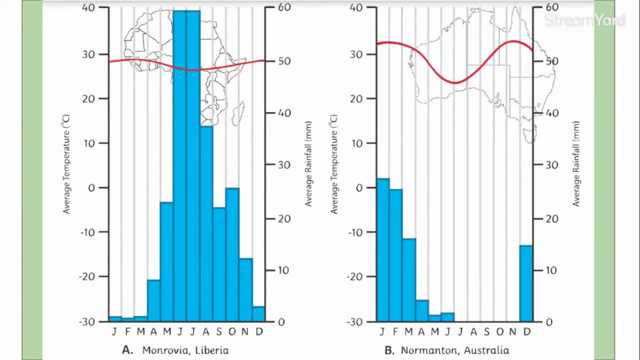 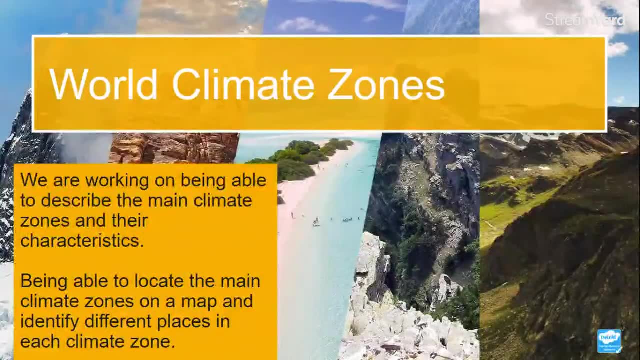 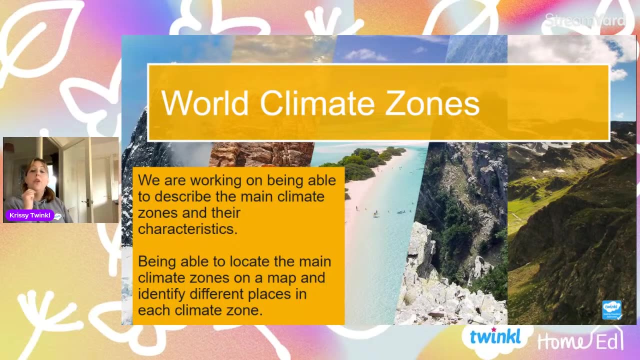 looking at all the different axes and you're looking at all the different lines and bars. it's really tricky sometimes to get to get. I can't get my words out. I need to go and have a lie down to get to read it accurately. So today we're going to be looking at climate zones. 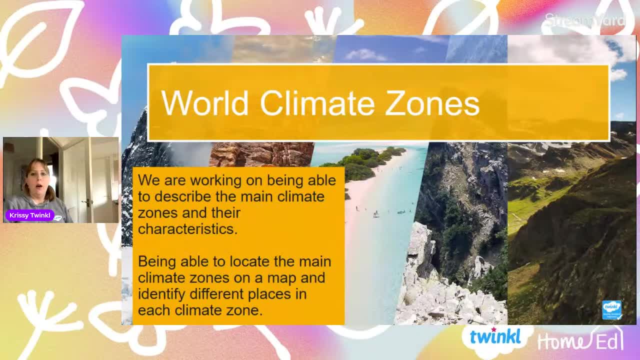 So we're going to look at what climate zones are, describing the main climate zones and what their characteristics are, and then I'm going to set you an activity to look at climate zones on a map afterwards, if you wish, and identifying different places in different climate zones. but before that, we're also going to do something a bit more. 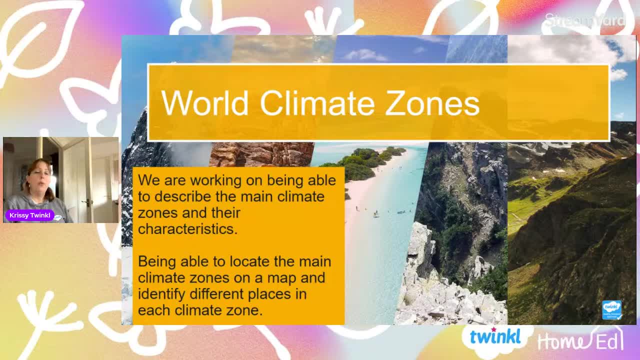 complicated, and what we're going to do is we're going to look at what's the difference between a climate zone and a biome, because this is a question I get asked a lot by GCSE geography students. Climate zone and a biome is exactly the same, because when you look at an atlas at the back of 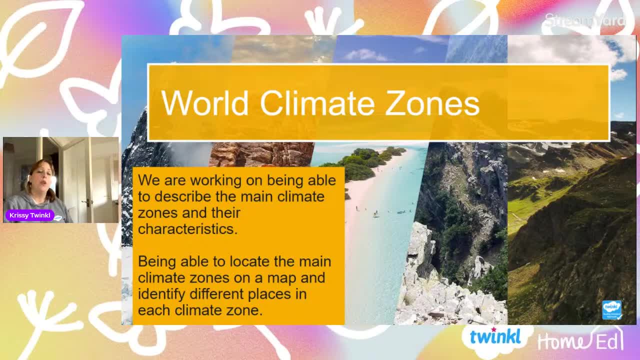 an atlas. if you've got a good atlas. it has lots of different world maps and it charts population and it charts climate and it charts biomes and it does all sorts of things- economic development- and we've looked at the different types of maps when we did map skills but we're going to look. 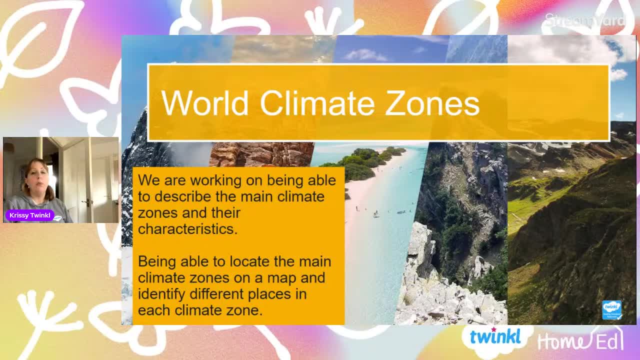 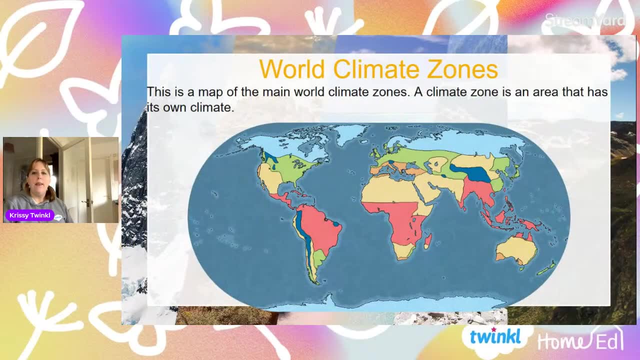 at what the difference is between a climate zone and a biome. Now, the reason that we're gonna do that is because sometimes people get a bit confused, so we're also gonna do that now. this is a map of the world's climate zones, and so a climate zone is an area that has its own climate. 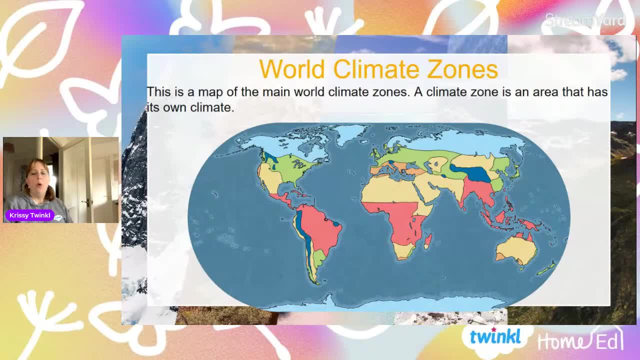 so all of those. so if you look at the red, if you go anywhere there, they have the same climate. if you go anywhere in yellow, it has the same climate. if you go anywhere in green, it has the same climate, and so on. and so that's how you. 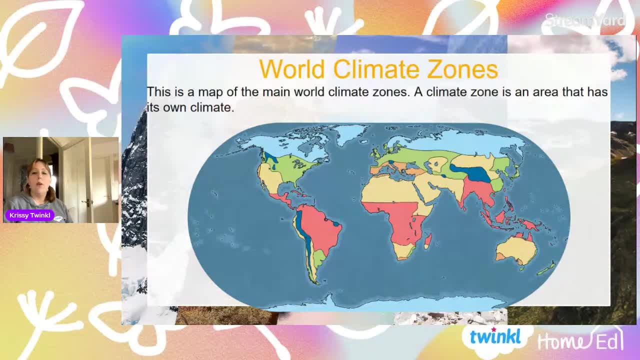 work. that's how geographers have worked out climate zones. now, a really important thing to say is that if you say, look at africa, it's not like an extreme line. so if i'm on the red side, i'm in that climate zone, and then if i slightly jump over an imaginary line, i'm in a different climate zone. 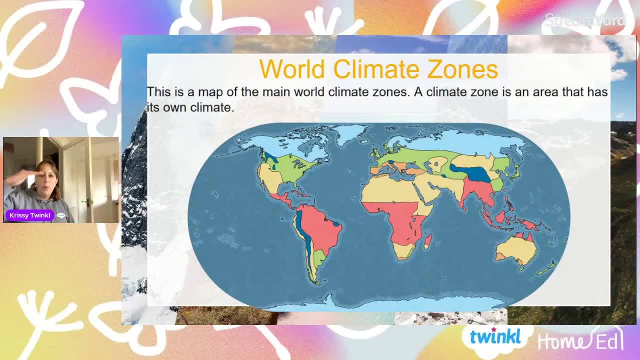 it's not as easy as that. the climate, where you've got those boundaries, the climate gradually changes, so it's not as extreme on in real life, but it's a pictorial representation of roughly the world's climate zones. but, as i've said, it doesn't mean if i'm stood on the right in africa, i'm stood on the. 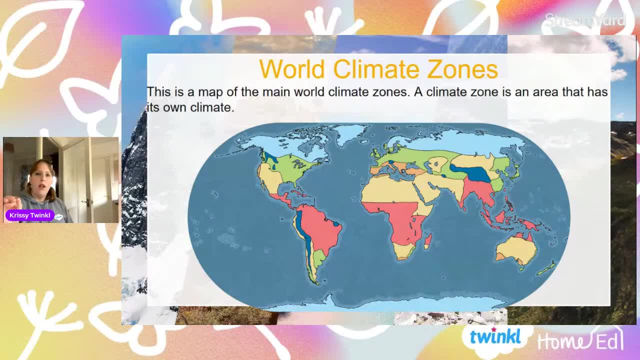 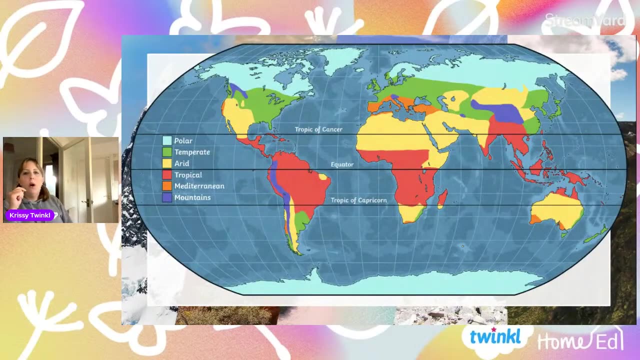 right in the right section, red section, and then i jump right a little bit and i'm then suddenly in the yellow section and i'm in a different climate. it's not that it's a gradual change, but these are roughly the different climate zones, and so what we have is we have, right through the middle of the 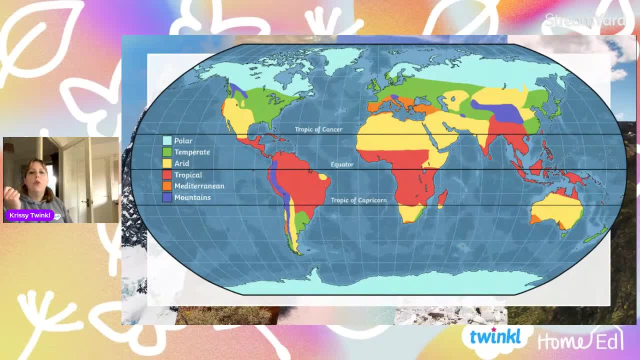 line. we uh, middle of the globe, we have the equator, and so if you look, as you look up, from the equator up, you'll see the climate zones going from red to yellow, to purple, to orange, to green to blue, and if you look the other way, you'll find the same. you'll go from kind of 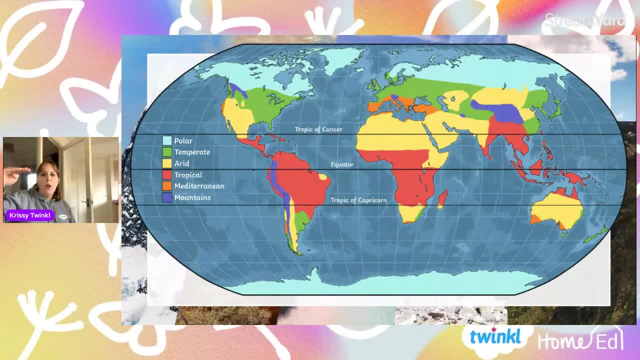 red to yellow to purple, uh, to orange, to green to blue. roughly loosely they do do roughly mirror, and so the blue climate is known as the polar climate, the green colors, so anything in green, is known as temperate, a temperate climate, and we, if you are in the uk, 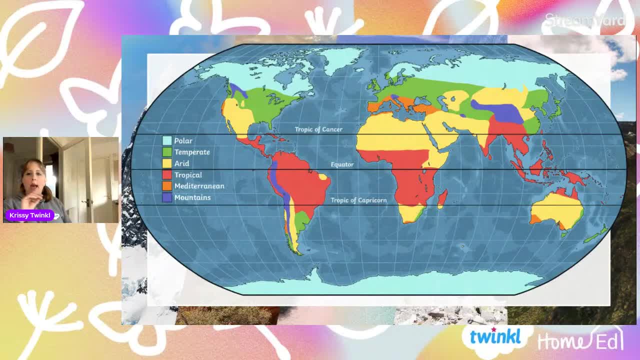 our climate is the temperate climate. yellow is arid, so the arid climate. red is the tropical climate. blue- i'm gonna go lie down, i can't get my colors out. orange is the um mediterranean climate and blue is a mountainous and we're gonna look at. it's not really a climate, the mountainous- but 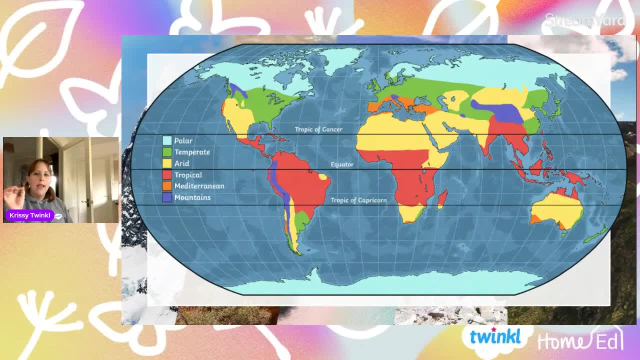 we're gonna explain why, so later. okay, now lots of you going on. it's to do with temperature. it's not just to do with temperature, it's to do with average temperature and average precipitation levels. uh, because, uh, and from that humidity. so there's a real, real important thing to say. it's 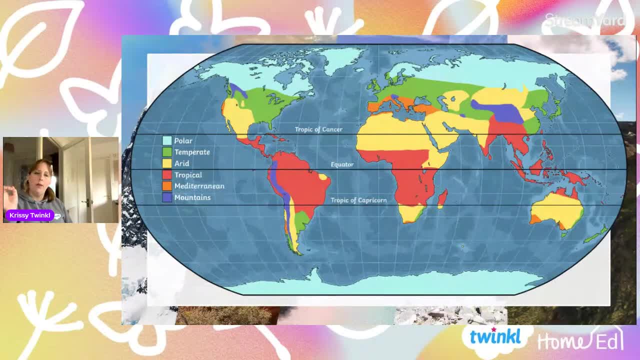 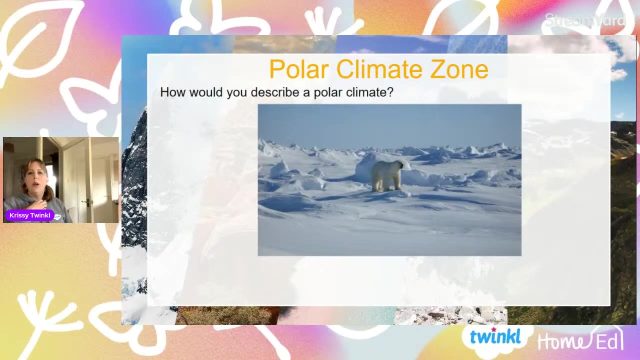 not just based on temperature, because it's a climate graph, so it's based on the average temperatures that those places see, the levels of humidity and the levels of precipitation. that's how it's worked, okay. so the first thing we're going to think about is the polar climate. 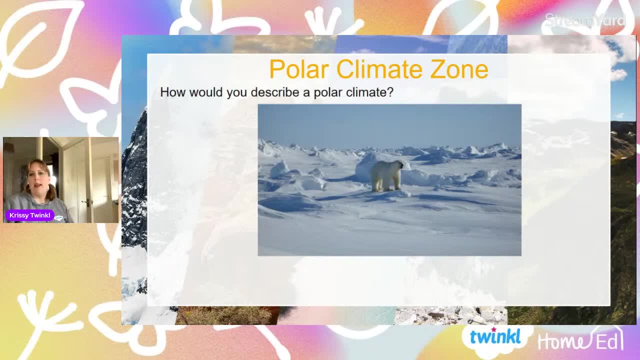 we're going to start off pretty easy. um, and that is how would you describe a polar climate? absolutely so. if you're thinking about mount everest, if you're at the bottom of mount everest, then the climate is going to be completely different. if you climb to the top of mount 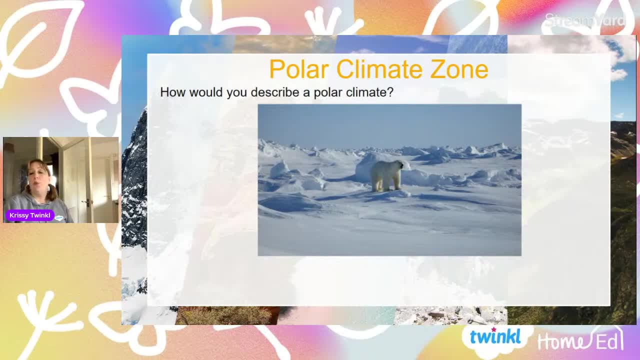 everest um and so uh. that's why, when they started to develop climate zones- well, hang on a minute- it started to develop climate zones. well, hang on a minute. it started to develop climate zones. well, hang on a minute, because you could be somewhere really really quite hot and arid, and then you'd climb up to top of the 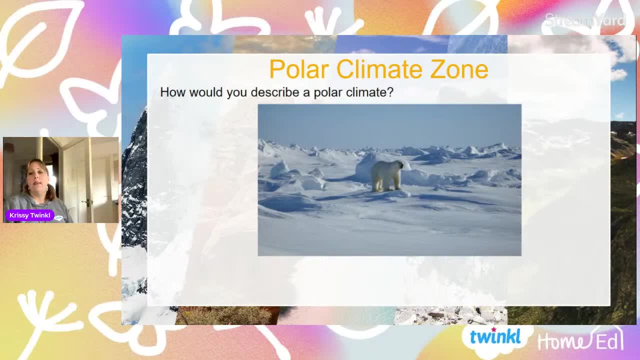 mountain and then it's freezing cold and there's snow, and that's exactly why we have mountains. so thank you for that. the closer you get to these imaginary lines, the two kind of yes, uh, whoever's behind that comment, yes. so the closer you get to these imaginary lines, the more you see those. 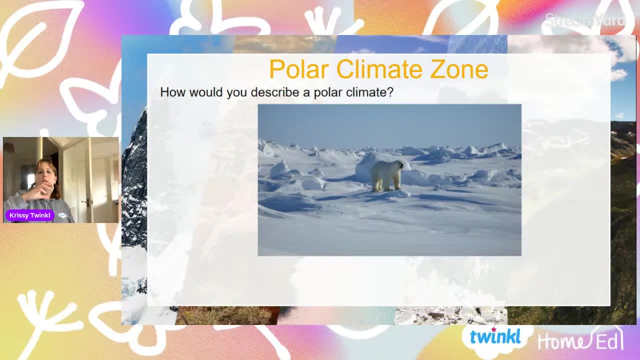 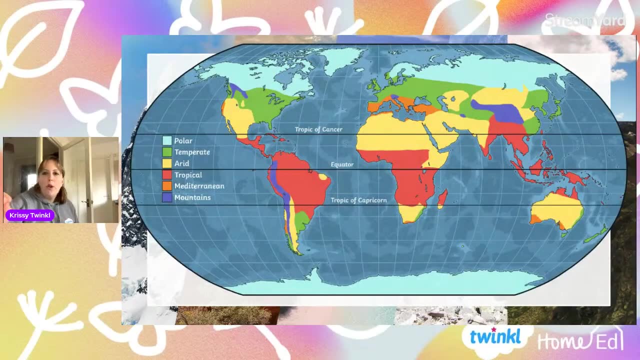 climates start to blur. so if you are in like a tropical climate where it's hot and and it's- if you look here, for example, if you look in south america where you have, um, the tropical climate, as you move forward it the rainfall starts to drop, so you basically are getting then the yellow. so 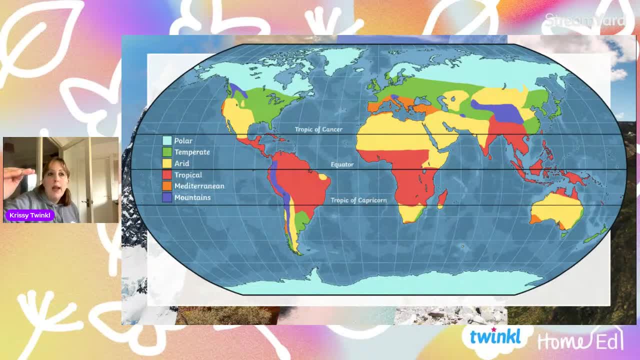 you're getting an area that's still hot but isn't quite as that isn't wet, and so you find these blur. but it's also this kind of goes in with next week as well, because there's also other reasons at play scientifically as to why this happens. it will make a little bit of a difference for the 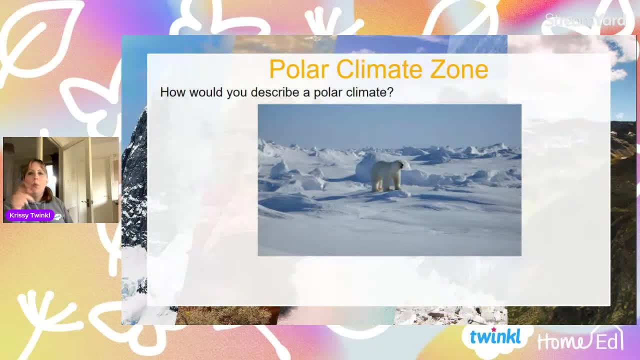 little bit tinier. more sense um, when you've also done next week, because there's other things at play. but yes, loosely, you're absolutely right. so we've got dry, we've got icy, we've got snow. minus temperatures. it's considered desert. uh, it's colder the higher you go, absolutely so. polar climates. 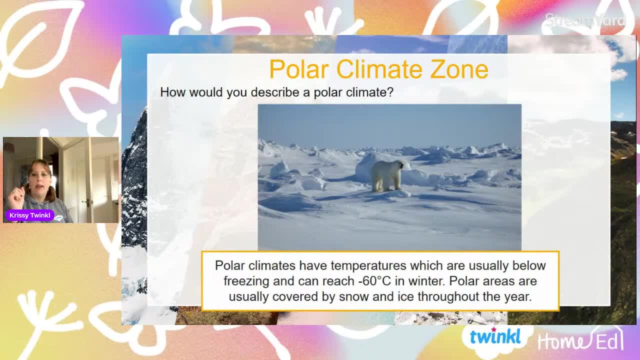 have temperatures which are usually below freezing and they can reach around about minus 60 in winter, and polar areas are usually covered by snow and ice. um, and so that is what a polar climate is. it's kind of, yes, considered a desert, but it's considered a desert for a different reason, and 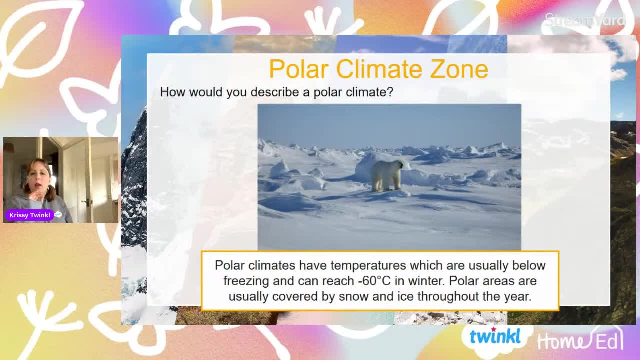 that's to more to do with biomes than climate, um, because nothing grows there. so we'll get onto that in a minute. but yeah, when you're looking at talking about it, the climate zone, not the biome, the climate zone, um, it is freezing snow ice throughout the 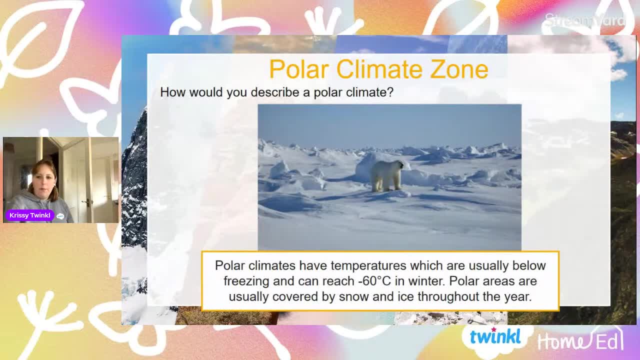 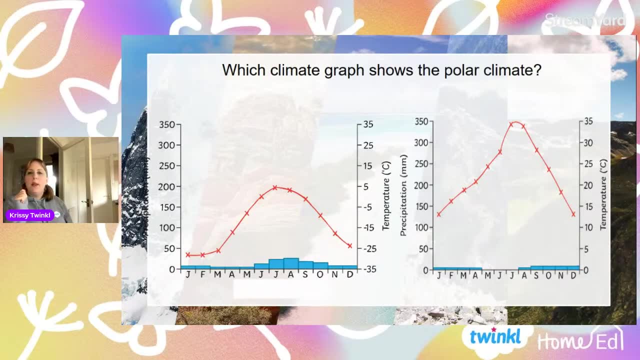 year and it's about minus 60. okay, no, tropical and mediterranean is not a desert. so which climate graph do we think shows the polar climate? so it's freezing temperatures um and um, not a huge amount of rainfall. you might want to start looking at, uh, these two climate graphs. which climate graph do you think shows a polar climate? 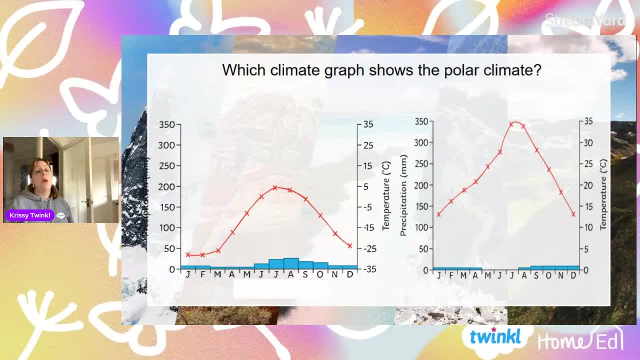 now you're absolutely right. the temperature does go up in both of them because you don't have in a polar climate the temperature isn't the same all year. you can see that actually the temperature still fluctuates even in a polar climate, and the rainfall slightly fluctuates. it's not a huge. 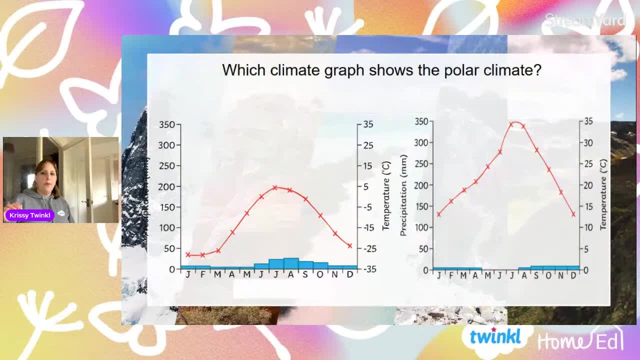 amount of rain, but the rain definitely also does fluctuate um and so, uh, there is definitely a climate, uh, there is definitely a temperature change, but you absolutely should have gone with a, because you can see that in a uh, you can see that the temperature uh is getting down to kind of minus 35 on that graph, so absolutely, 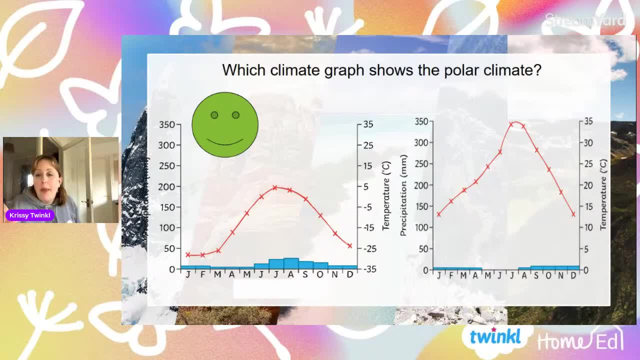 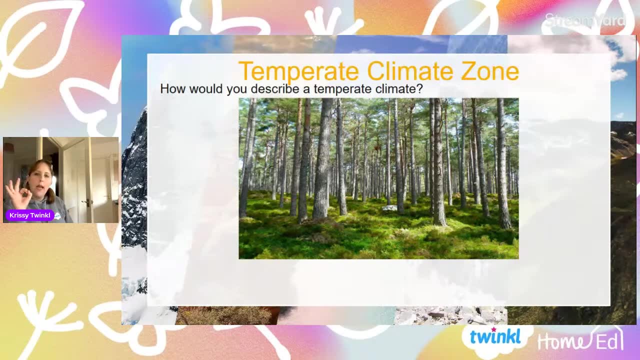 you've got that roughly, uh, correct. so that that's a polar climate graph. so we're only talking about the climate. i don't want to hear about the trees, the vegetation, the animals. i just want to hear about the climate. so what climate would you see if you were in a 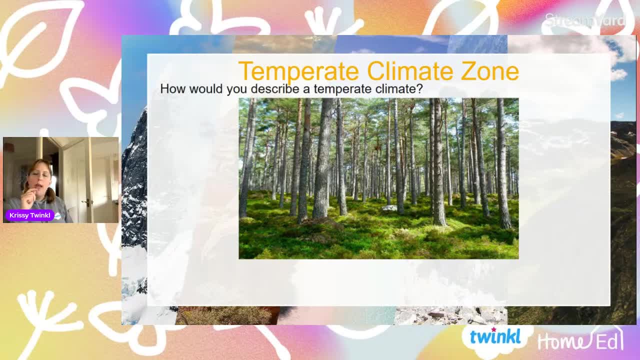 temperate climate, because we, if you're in the uk, we have a temperate climate. so what does a temperate climate mean? and it's more tricky than just saying it's cold all year, either slightly cold or like seriously cold. it's a bit more complicated, so think about. 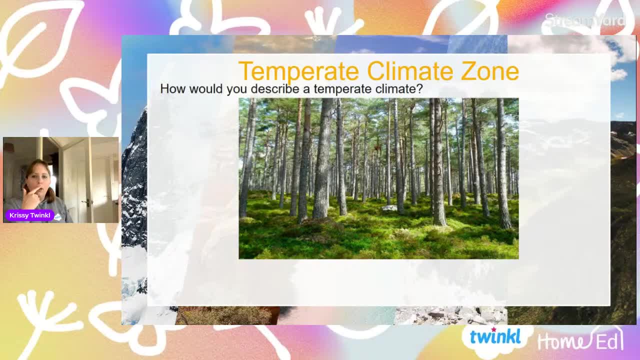 the temperature, think about the rainfall. is it warm? because we're in a temperate climate right now and i can guarantee you i'm not warm. it's minus six where i am today. um, so i don't think that that's quite right. your news: warm summers, mild winters, absolutely steady rainfall, do we? 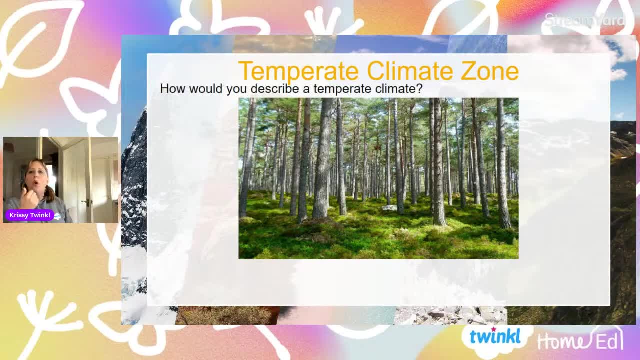 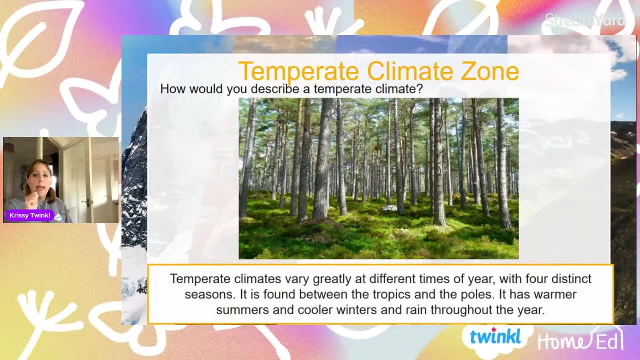 have rainfall all year, steady, so is it warm in the summer, colder in winter, seasonal rain, warm and cold, can't make its mind up sometimes, where it has four seasons. so, yeah, you're right. so the temperate climate is a climate that varies greatly to the different times of year, so we have four distinct seasons, and that's something you 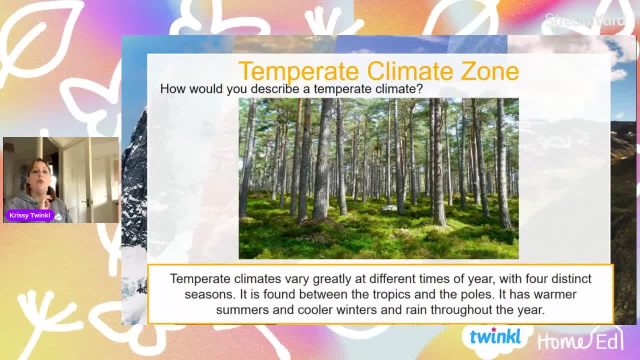 really need to understand when you're looking at climate zones. other climates do not have clear distinct seasons, but we have four distinct seasons. so we have four distinct seasons, and that's we do. we have four distinct seasons: spring, summer, autumn, winter. but if you go to another climate, 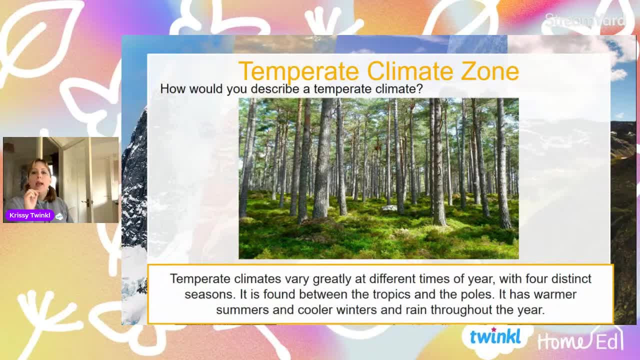 zone. some plants don't have any seasons. it's found between the tropics and the poles and, you're definitely right, it has a warmer summer, a cooler winter. it has rained throughout the year and we have sometimes, but not always, more rain in the spring and the autumn period than we do in the 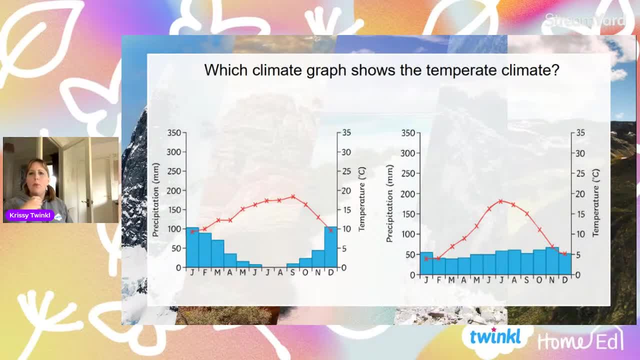 summer, but not necessarily always so. which climate graph shows the temperate climate? what do we think? what do you think is the correct climate graph? do you think they look quite similar, don't they? we've got some. we've got jack saying he thinks the first one. 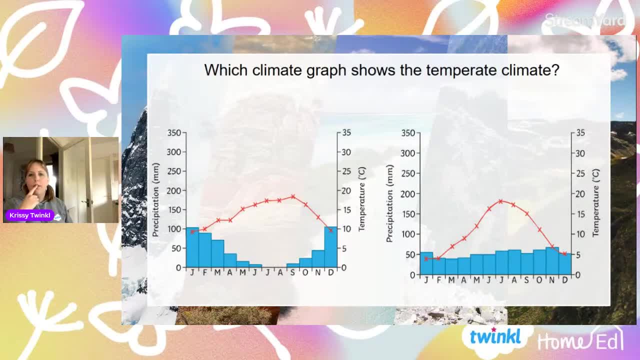 the first one. lots of you going for the first one got some b, a or b. oh, a bit confused, aren't we? it's actually b now. the telltale sign of this one is the rain we don't. we do have rain in the summer. if you look at the climate graph on a, it's telling. 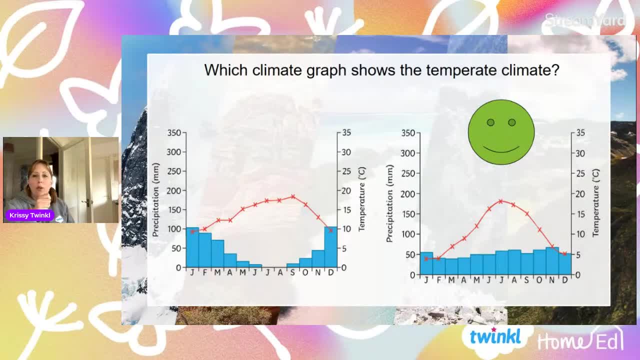 us that there's no rain in july and it's still there. so just remember, there is no rain on july and there's no rain in August. now I can guarantee you that we have sometimes rain in July and in August. if you look at it, we have pretty. if you're looking at the climate, we have pretty roughly. 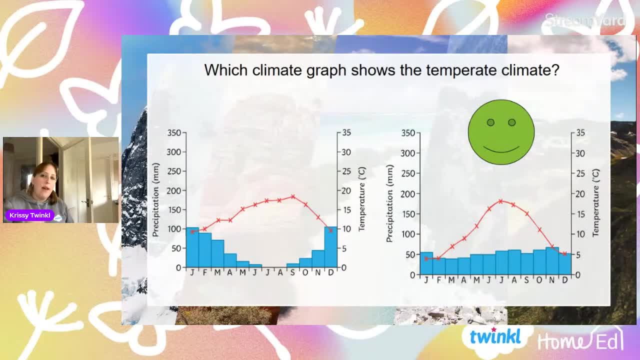 pretty steady rainfall throughout the year. because you're looking at that average, don't forget now, although we're getting progressively warmer in the summer and we're having lots of times where we have a shortage of water and hose, pipe bans and all those things, actually in the last 30 years the rainfall isn't that much different throughout the year. so if you've got B, 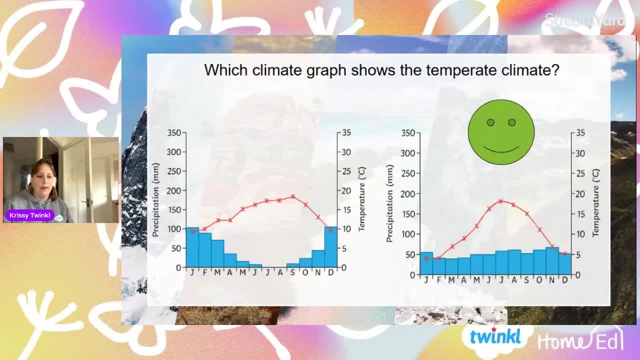 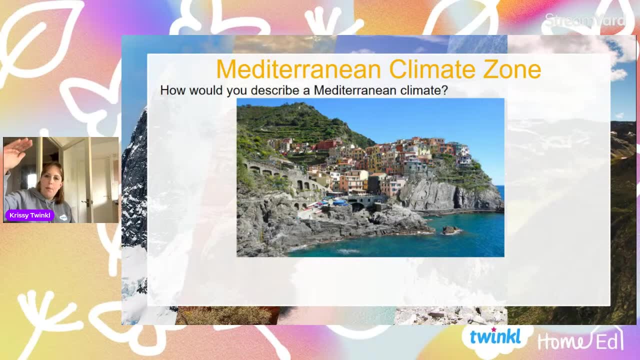 well done, because we definitely do have rain in July and August, sadly. now the Mediterranean climate zone, so, as you get more down from the temperate, more into the Mediterranean- so we're thinking about the south of France, places like that- um, um, um, what do we think? how would you describe the Mediterranean climate? because it's not. 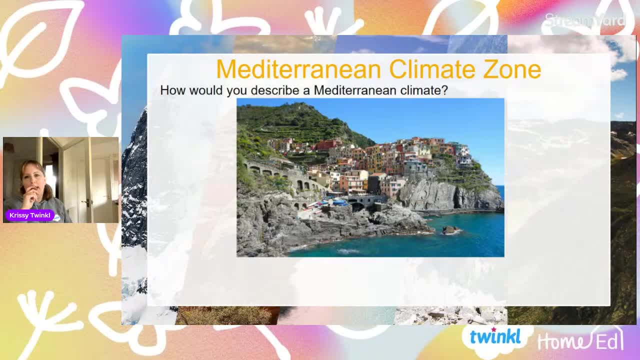 significantly different to the temperate climate zone, is it? if I go to the south of France now, what would I see? what would make it different from what we're experiencing right now? what do we think okay, warm when? so there's somebody saying dry, hot summers, no rainfall, but warm summers, cooler winters, a bit wet. 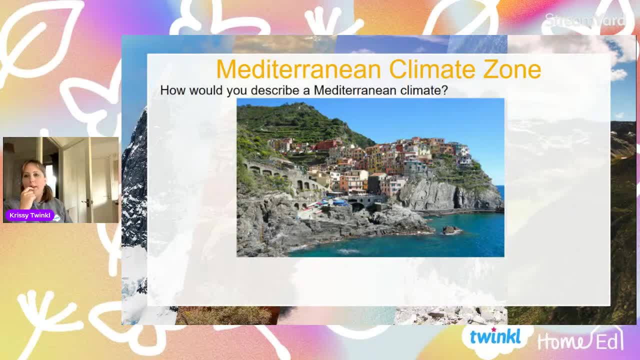 choose to review it absolutely. that's where I am now. it's six degrees. so there we go. where there's a that comment Cloemy's family. so if you're 6 degrees in the south of France, we're minus six degrees, so that is a difference between 12 degrees. I really wish I was with you because my, my temperature, my outside, 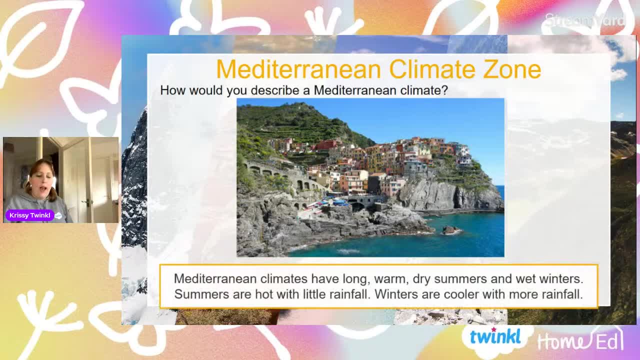 temperature, but my garden says it's minus 6. so you're absolutely right. they have long warm, dry summers, but they still do have wet winters, so they have hot summers. you're going to find them when they get warmer but, by the way, most in the southắc. 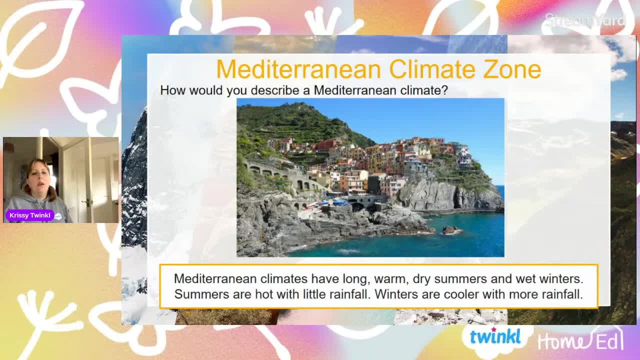 you have long warm, dry summers, but they still do have wet winters, so they have hot summers. we've seen some covidD winters, so they have hot summers with little rainfall. winters are slightly cooler, with more rainfall, so you still get those seasons and those temperature changes, but they're less extreme as 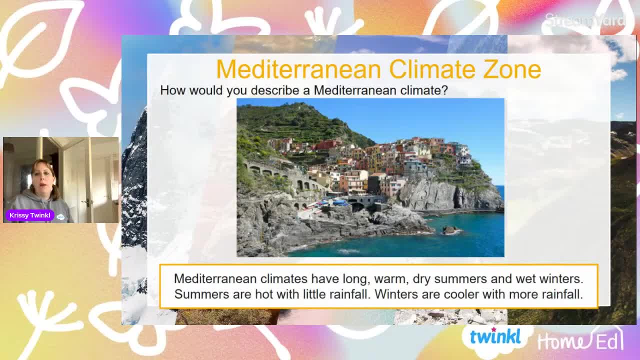 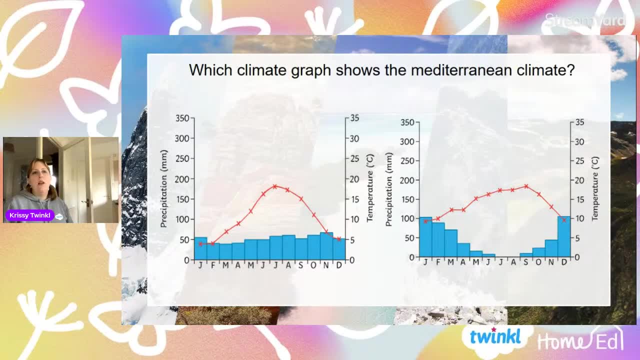 they are in the tempera. so, oh north spain, can i come and do my lessons with you guys, because it sounds a lot warmer over in there? so yes, the mediterranean climate is slightly different to the tempera in respect of the fact that they have warmer, drier summers. what climate graph. 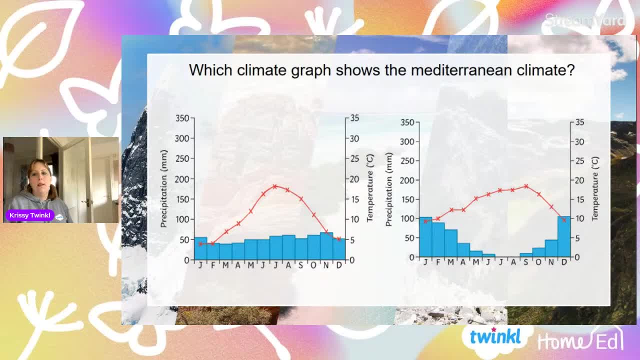 therefore shows the mediterranean climate. which one do you think to have a little look? which one of those is the mediterranean climate? what do we think? do we think it's the left or it's the right? what do you think henry's going for? b? 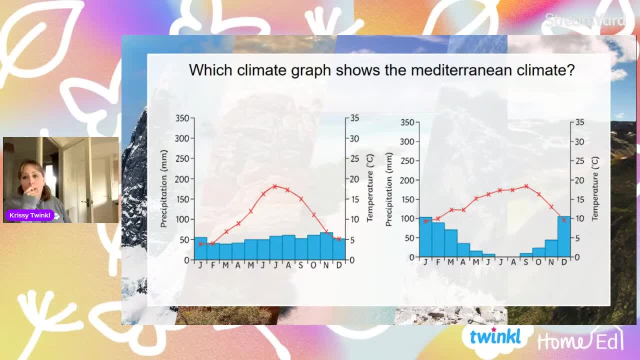 well, i don't know where you are. in england there's three degrees minus six. when i let my dog out this morning, minus two here. so yeah, what about the mediterranean climate? you're definitely right, it is b, because you can see that dry season in july and august. 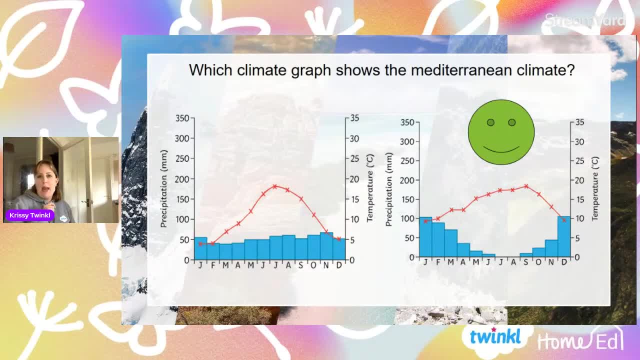 and that's why often we tend to go to on holiday to spain or portugal or italy, because they are part of the mediterranean climate and that's exactly the point. so someone's saying they're in. i'm talking about this blurring of those climate zones. if you're in north spain, you'll find that. 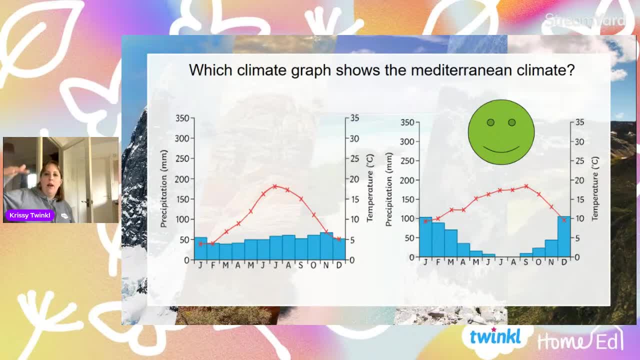 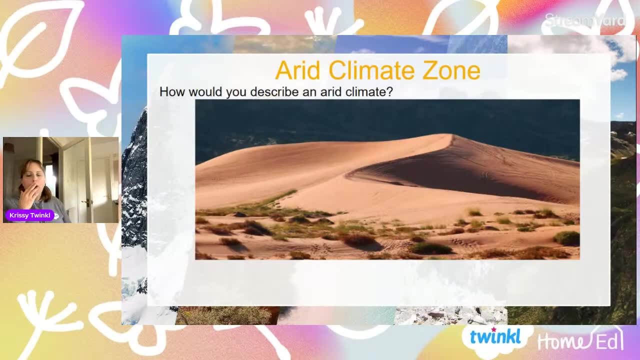 you have a slight mix of temperate and mediterranean, so there's sort of little, a little bit of a mix there. okay, arid. so what do you think? an arid climate zone is an arid climate. so this is a picture if you're unsure what the word arid means. so what do you think? an arid climate? 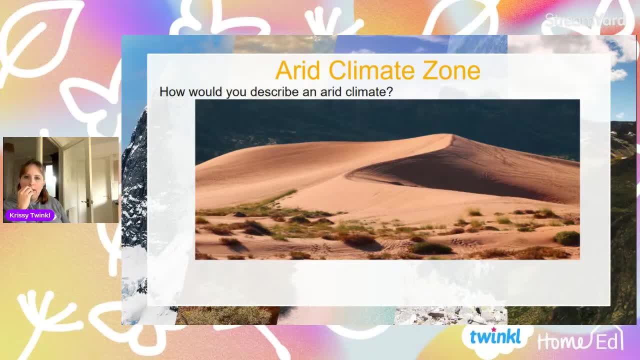 is like. what do you think arid? look at it. it's an arid climate zone that looks dry and hot all the years. you think is it very dry all the year? do you think it has very, very warm and dry during the day, freezing at night, no rainfall. so what do we think arid? interesting. 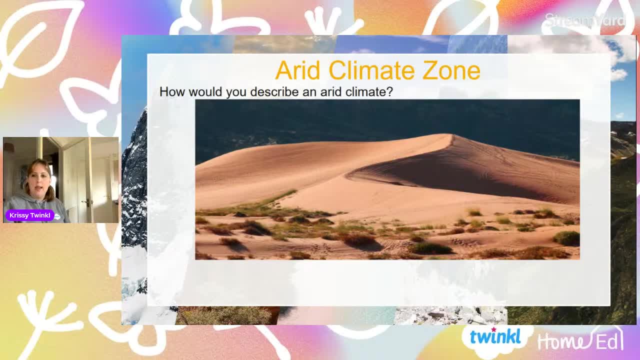 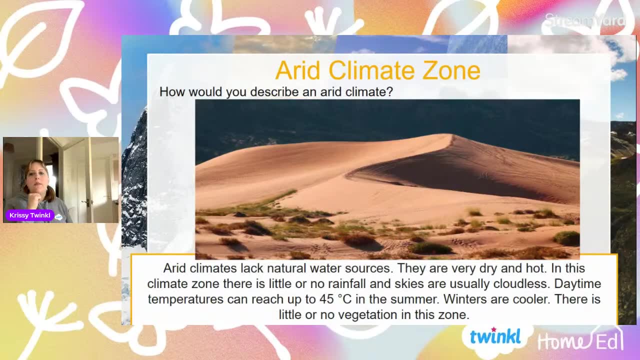 no seasons, lots of dry, lots of really good answers here. so an arid climate lacks natural water sources, so they're very dry, they're very hot and there is little or no rainfall. and if you go to an arid climate zone and you look up into the sky, they are usually- it's usually- cloudless. 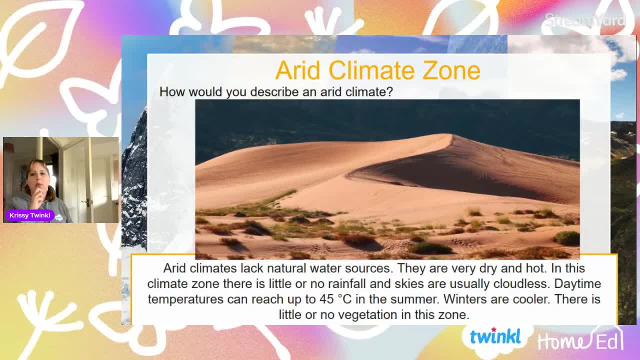 now, daytime temperatures in an arid climate zone can reach up to 45 degrees, so it is really really warm. but in answer to the do they have no seasons. you can find that winters are slightly cooler, and definitely in arid climate zones, dependent on where, you can find that the nights are very cold. 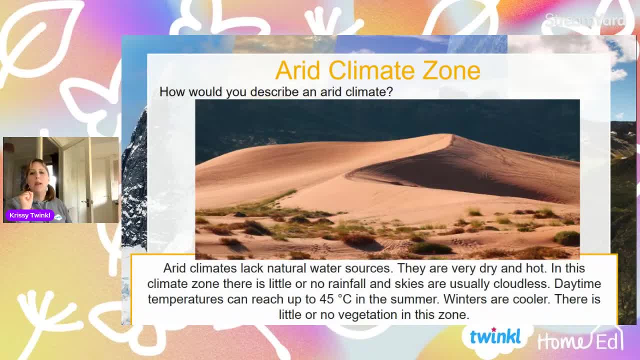 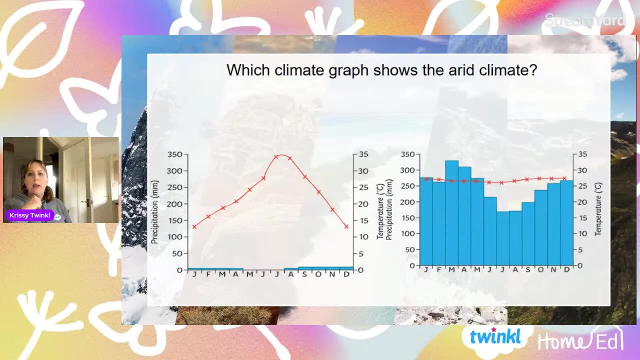 because there's not a lot of vegetation to hold the temperature in. there's little or no vegetation in this zone. so, yeah, our climate zones are really dry and really hot. so then that leads me to these climate graphs. shows the arid climate. which one do you think the arid climate? 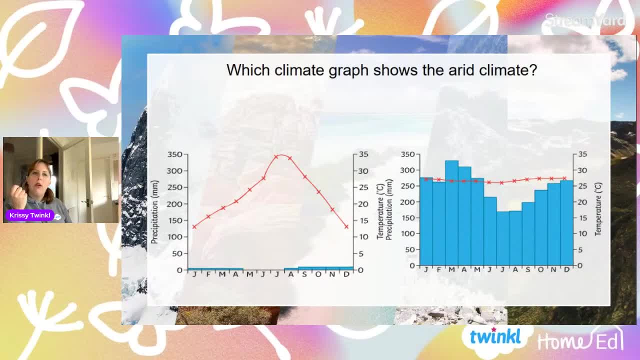 so places get cold in arid climates if they are where there's not. you know, if there was no buildings, there's no uh rocks, there's no vegetation and the air is absolutely nothing to hold the heat. it will get colder at nights and you're absolutely right, it's definitely a that is. 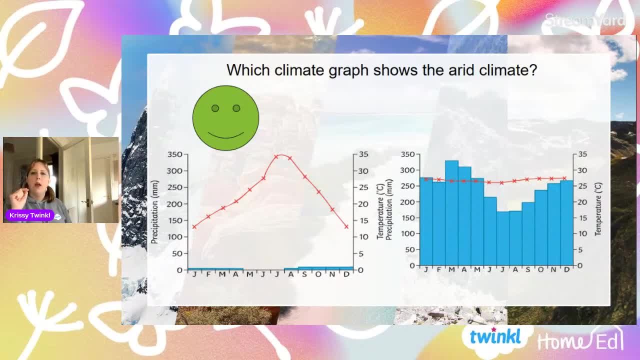 sun and rain. can you see this here? minuscule amount of rain, but can you see that the temperature does alter. so there is a slight season there. you've got like cooler months and then you've got really hot months. so, although you wouldn't call it a specifically clear seasons, it's not the same temperature all year, so certain. 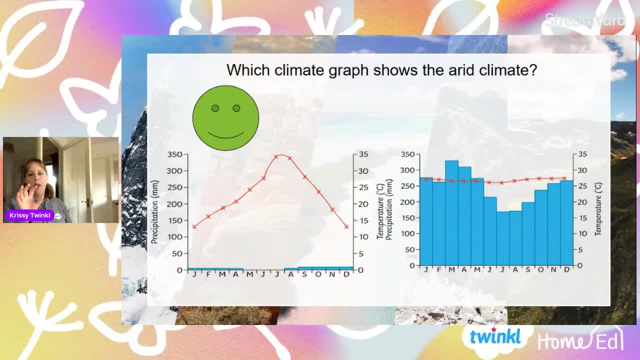 times of the year it's cooler, other times of the year it's hotter, it's not hot. if you look at the climate graph on the right, then you see the temperature is the same all year. so it's not quite the same as that. the arid climate. the temperature does change, right? the next one, the? 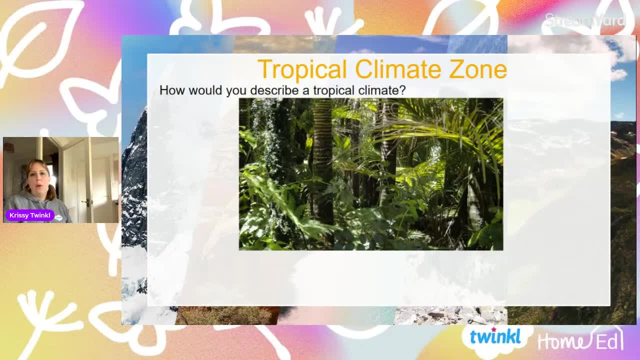 tropical climate zone. what is the tropical climate zone going to look like? and remember, we're looking at climate. so what do we think the characteristics of a tropical climate zone would be? so peru and brazil. yet they have a tropical climate zone: absolutely hot and humid, a rainy season and 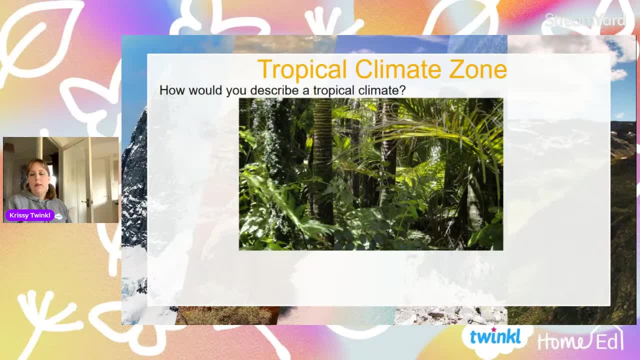 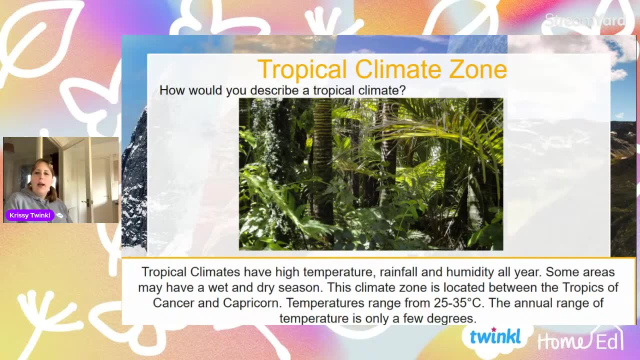 a drier season, warm and humid, sunny, wet, awesome, absolutely so. tropical climates. they have high temperatures, high rainfall and therefore, as a result, high humidity levels, so that sort of feeling where you get all sweaty and all your clothes stick to you. they do, or they can have a wet and a dry season, dependent on which particular area of the world you're going. 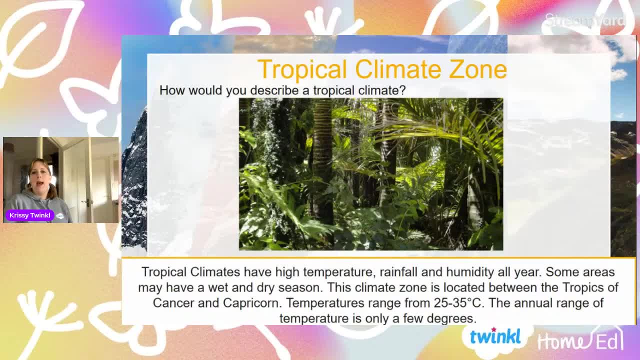 with the tropical climate zone. you'll see a slight difference in that, but they may have a wet and dry season, and the climate zone of the tropical climate zone is found between the tropics of cancer and capricorn, and the temperatures range from 25 to 35 degrees dependent on where the 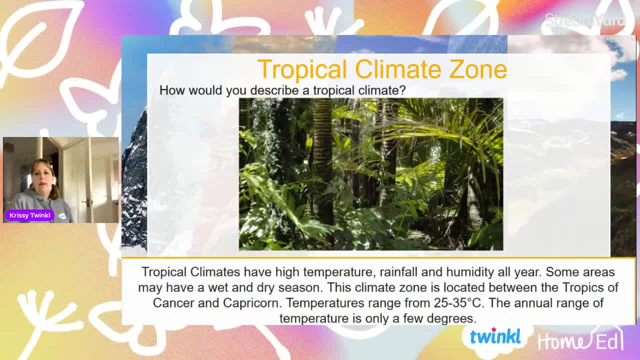 tropical climate zone is and- and the biggest thing about this is that there isn't any seasons- the average, the annual range of temperatures. you're only seeing a slight change. so, whereas we can be minus six right now, but in july we might be 28 degrees, that is a huge variation in temperature. but tropical climate zones, their annual, 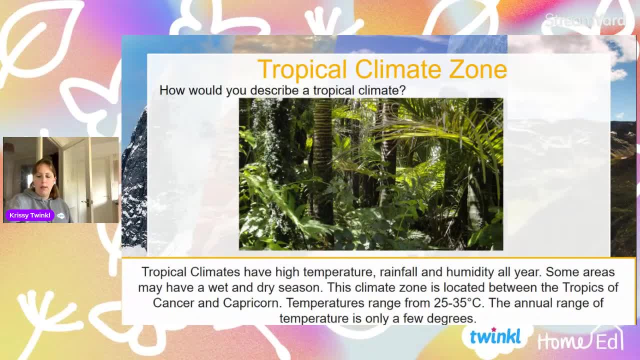 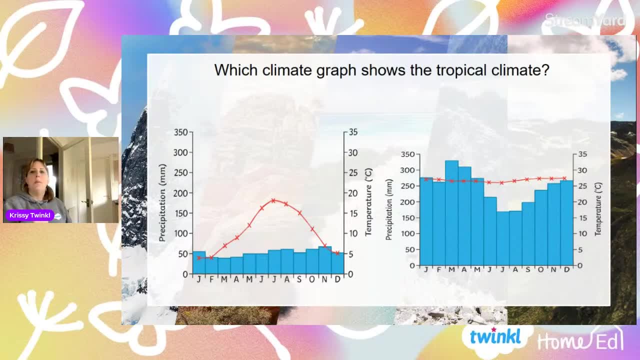 range of temperature is very minuscule, only a few degrees. so you'll find that the temperature pretty much stays the same. so that leads us to this next one. which climate graph here shows a tropical climate? do we think it's the left one, or do we think it's the right one? and how do you know? how do you know we're? 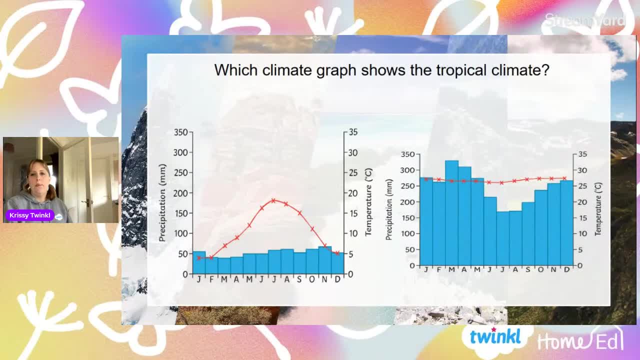 gonna go for b? how do we know it's b? someone's saying a? how do you know it's a? what's the big thing about tropical climates? the temperature doesn't really change. so which one's showing the temperature not really changing? absolutely it is b. so if you've got b, it can't be b and a, because they're both completely different. 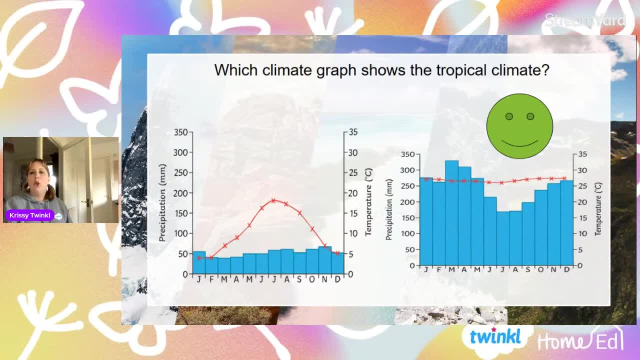 um, but it's definitely b because there's lots of rain. you can see that there is significantly more rain than if you're looking on the other side. so we've got precipitation up to nearly 350 millimeters, which is massive rainfall um, and the temperature is hardly moving. there's hardly any. 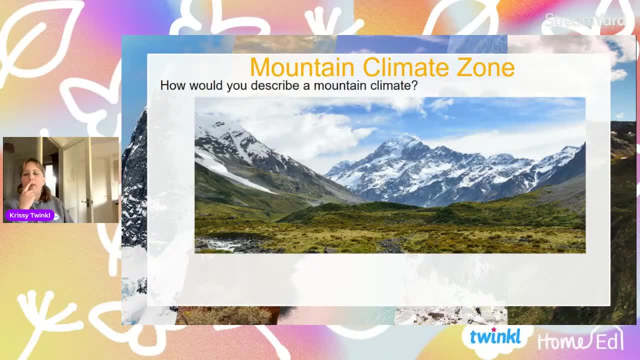 temperature change. so, absolutely right, a mountain climate zone. how do you think you'd describe a mountain climate zone? we have climbed a mountain. how would you describe a mountain climate zone? what would we think? mountain climate- what do you think? cold at the top. do you think all mountains are the same temperature on their altitudes? warm at the bottom. 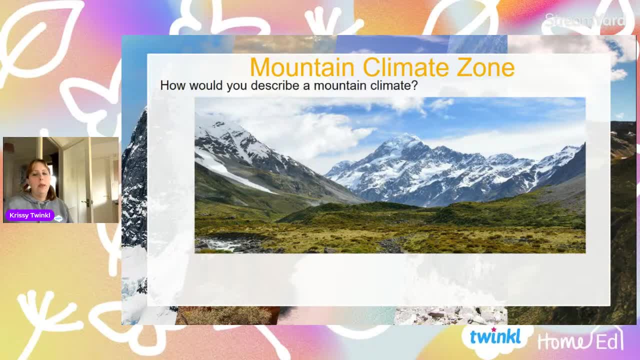 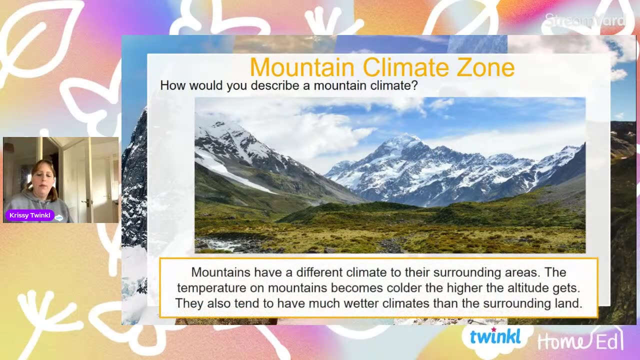 maybe depends on where the mountain is, vary climbing climate depending on elevation. really good, really great ideas. right now, mountains have a different climate to their surrounding areas. so basically, the higher you go up a mountain, the colder it gets, so that's a good idea. so if you go up a mountain, the colder it is because of the altitudes, and the higher the altitude the 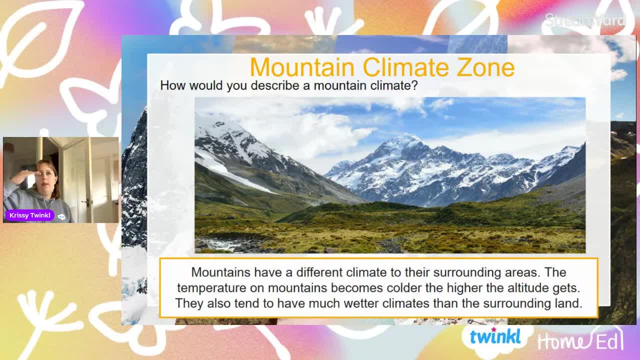 cold. you're going to find it, and so if you go, if the mountain is a significantly high mountain like everest, then you are going to find that as you are climbing the altitude, it's going to get colder and colder, and colder and colder. they often tend to have much wetter climates in the surrounding area. 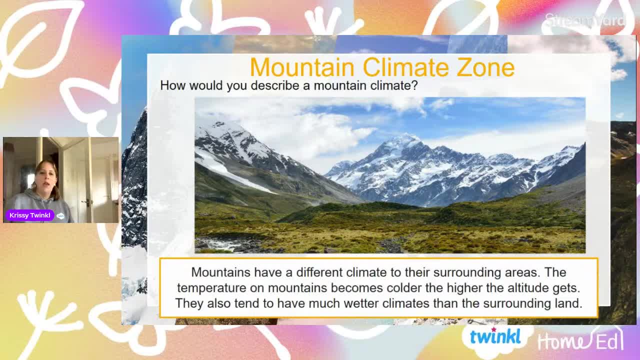 and the reason for that is also to do with the altitude. now you can't really distinguish a mountain climate zone with a mountain climate zone climate zone in terms of. they don't have- I don't have- a climate graph for a mountain climate zone, because you will find that the actual average temperatures will differ dependent on the mountain. 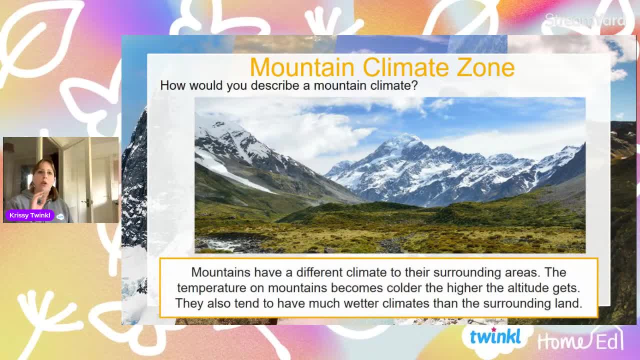 because it depends on the altitude of the mountain. so if you're looking at all the mountains around the world, they're all different heights and therefore the average temperature that you would have at the summit of one mountain is going to be completely different to the average temperature you. 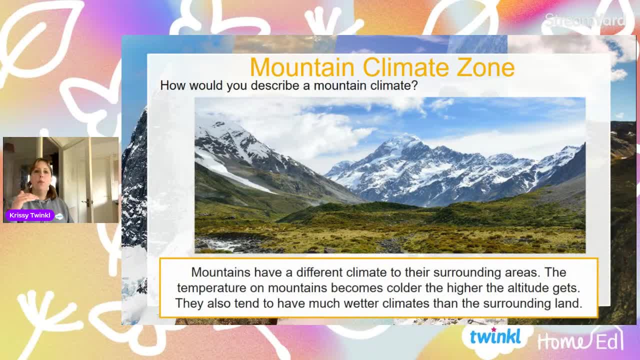 would have on the summit of another mountain, because that would be much more than a mountain mountain, because they would be different in altitude. But the reason that we distinguish mountain climate zones on on a climate world climate map is because that you will find they are completely different. 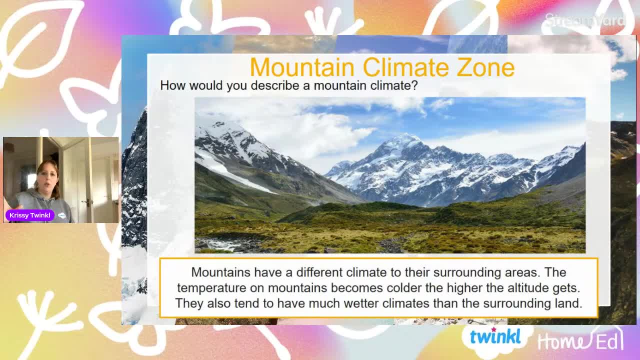 So if you have a mountain range going through your country, if you think about the Alps going through a Mediterranean climate like it, on the top of the Alps, I am not going to be in my swimsuit having a sunbathe because it will be significantly colder. 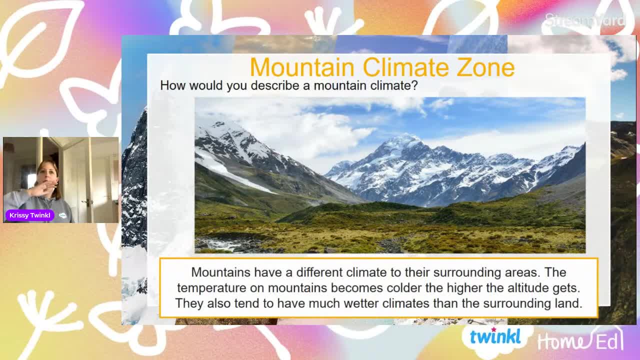 So I don't have a climate graph to show you, because you can't just blanket say what a mountain climate zone is like for average temperature, humidity and rainfall. It's about illustrating the fact that if you are in a tropical climate or an arid 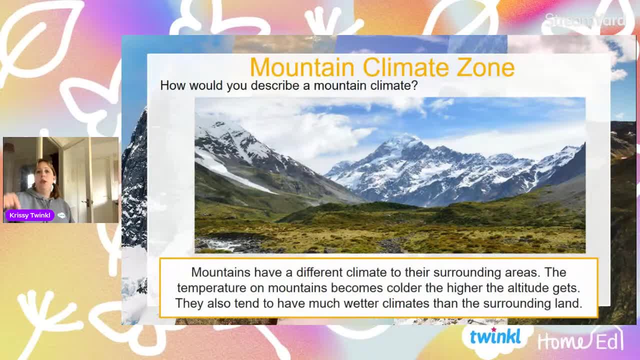 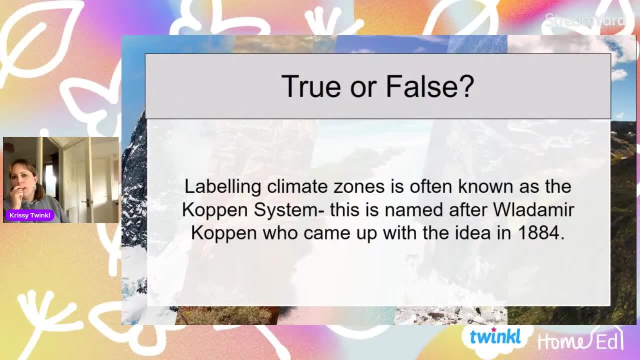 climate or a Mediterranean climate, and you decide to climb a mountain, the climate will be different. Does that make sense? I hope so, So let's play true or false. The concept of labelling these climate zones is often known as the Coppin system. 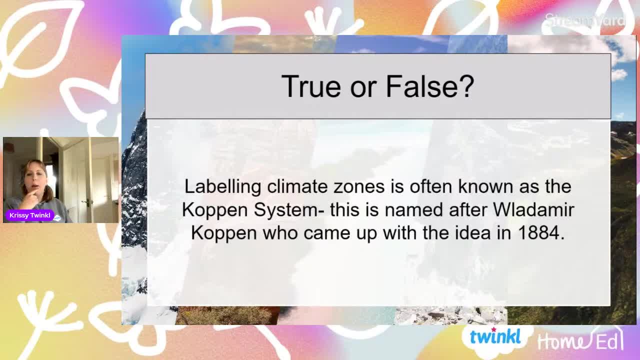 And this is named after Vladimir Coppin, who came up with the idea in 1884.. So what do we think? Do we think that geographers have been drawing climate maps till 18 since 1884?? Do we think that Vladimir Coppin came up with the idea? 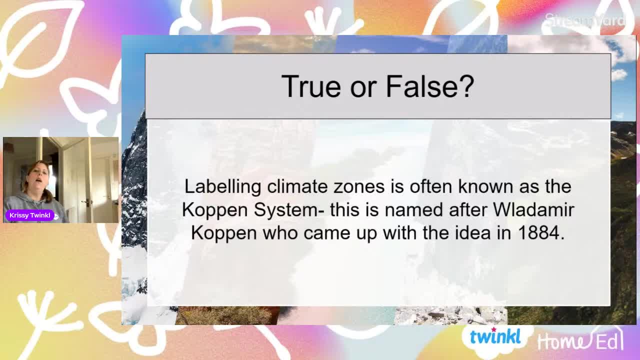 So if you see a climate graph, can you say, oh, that's the climate map. rather, You can say, oh, that's based on the Coppin system. What do we think? It's absolutely true. So you can say that if you see a climate map that's based on the Coppin system. 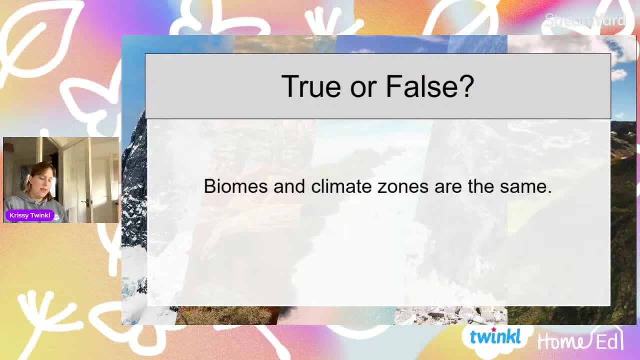 Now biomes and climate zones are the same. because I've seen this. now, This is exactly why I wanted to do this, because I've seen this as we've gone through. So as soon as I put up the arid climate, you went: oh, it's a desert. 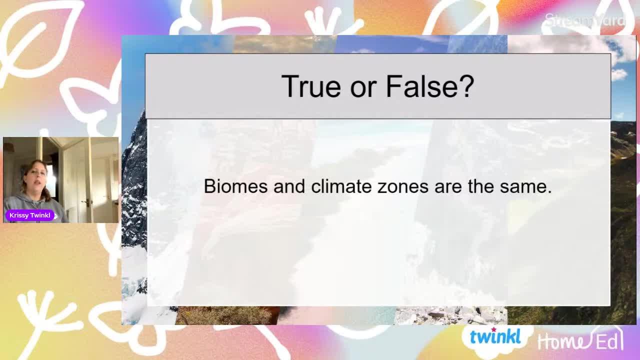 And as soon as I put up the tropical climate zone, some of you went: that's a rainforest. Now, is that meaning, therefore, that biomes and climate zones are the same? Because if we're talking about biomes, a tropical rainforest is a biome. 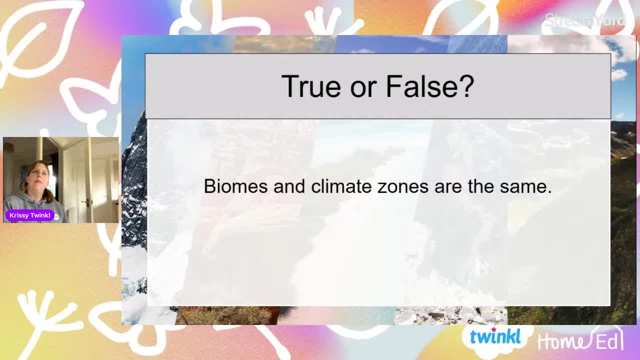 So if I look at a rainforest, a rainforest is a biome And if I look at a tropical climate, it's the same thing, isn't it? Is the biome and the climate zone the same? They're not. They're really different. 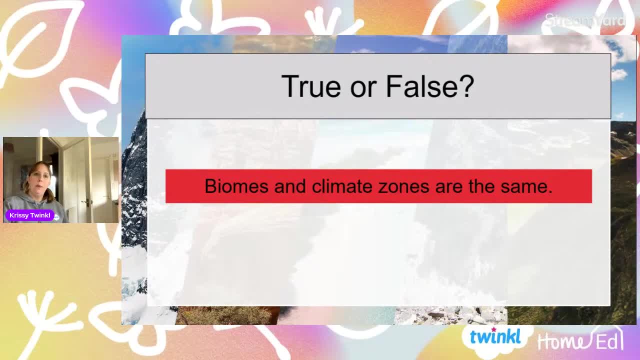 And it confuses people. and it confuses people because you look at a climate zone and you think, oh, that's the same as the biome. And lots of you did it. Lots of you started to talk about, oh well, it will definitely be like this: 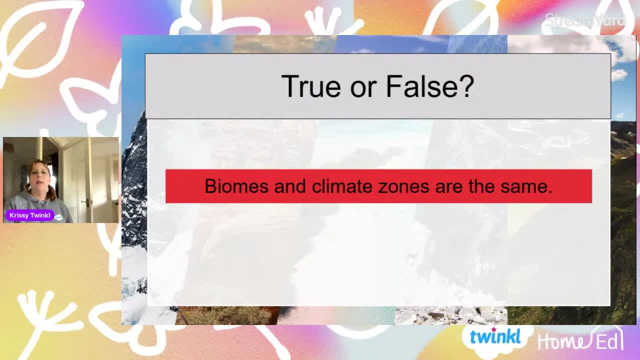 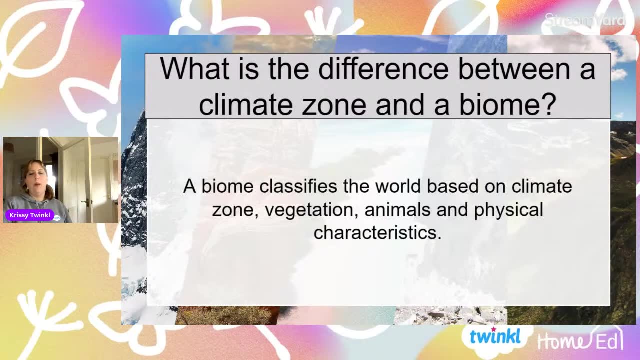 There won't be any vegetation growing in an arid climate zone because it's a desert. So we do it all the time, But they are actually different And this is the difference When we are sorting out the world to do with biomes. 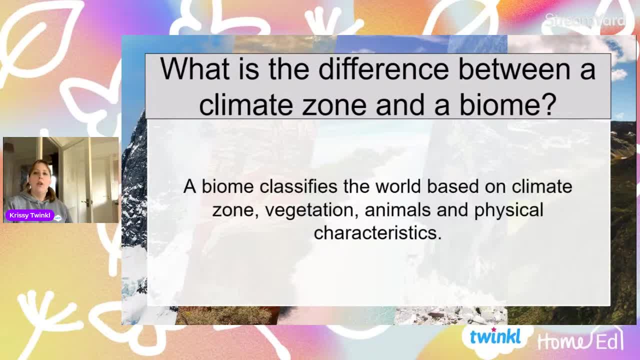 you classify a biome based on the climate zone. So the climate zone is a consideration of a biome, But you also look at its vegetation, You also look at its animals and you also look at the physical geography that you can see its physical characteristics. 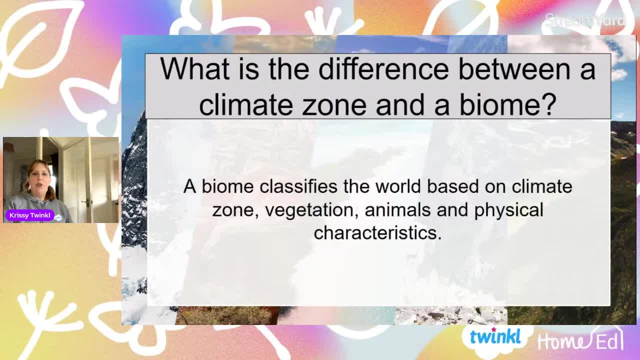 So they are Very different, But we tend to think sometimes that you can interchange it so you can go: oh, there's an arid climate, that's a desert, but it's not that different. A biome is classified based on the climate zone and the vegetation. 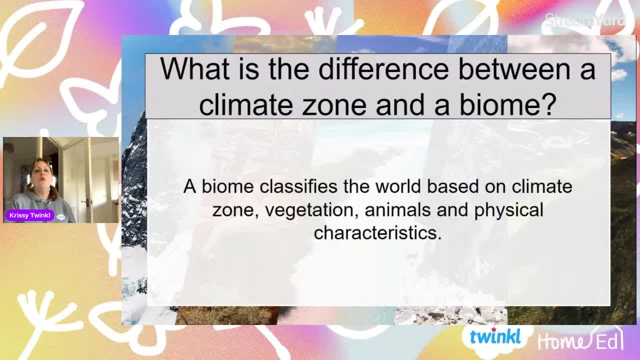 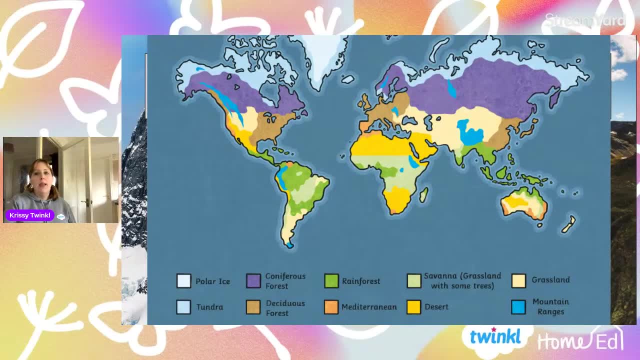 and the animals you would find and the physical geography that you would see. And so when you're looking at A biome It's completely different, But there is a little bit of overlap because obviously they are going to look similar, because when you're classifying a biome you're using climate as one. 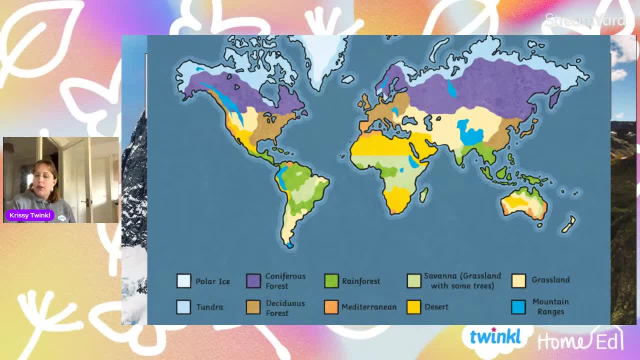 of the indicators, but they are different, they're not interchangeable And it's really important that you understand the different ways of talking. So, when you're talking about a rainforest, you're talking about the biome, You're talking about its vegetation, the animals, 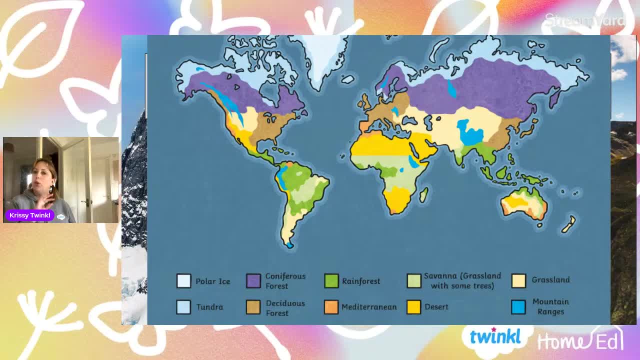 the physical geography and the climate, And so when you're talking about a rainforest, that is completely different to talking about a tropical climate. A rainforest has a tropical climate, but they're not interchangeable, And you can see that if you start to look at comparing these maps. 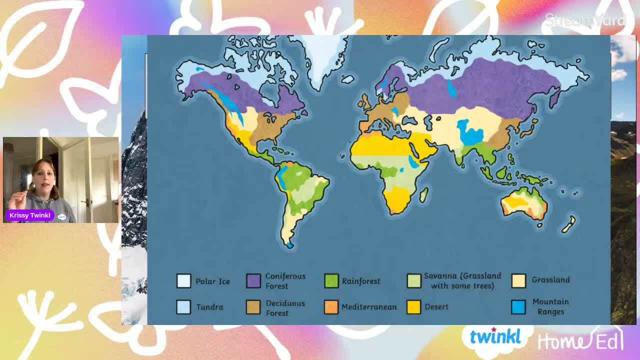 because you'll find that we have grasslands and we have deserts. So when you're looking at, for example, Africa, go and compare the biomes with the climate, because when we look at the climate graph, they do slightly differ. 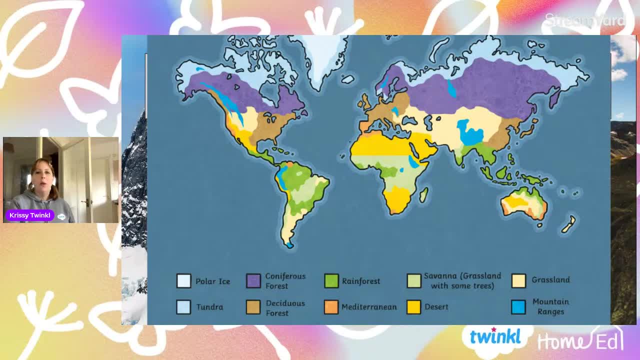 So what's why? Maybe go and have a little look. but you have deciduous forest. So our biome- if you are in England or the UK, our biome is deciduous forest, But our climate zone is temperate. Does that make sense? 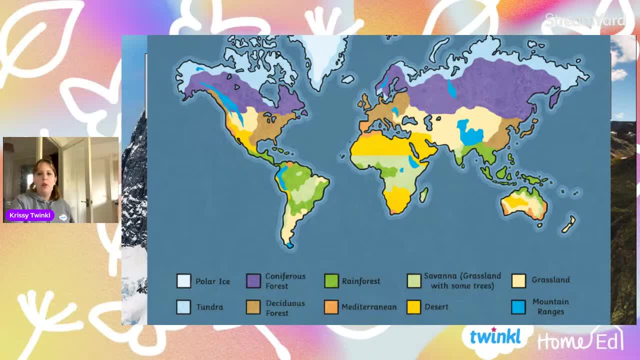 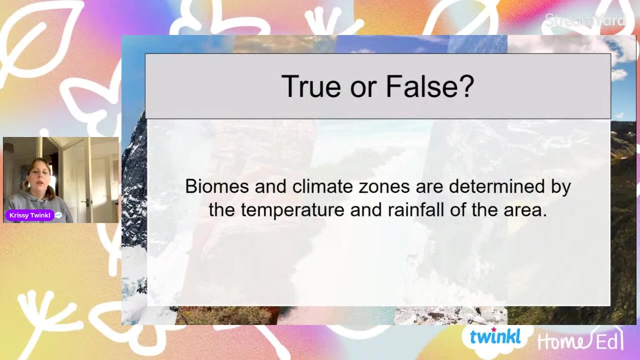 But it's really important that you understand that these things are not interchangeable, because if you look at savanna and grasslands, for example, they are slightly different biomes but they might have very similar climates. Does that make sense? Biomes and climate zones are determined. 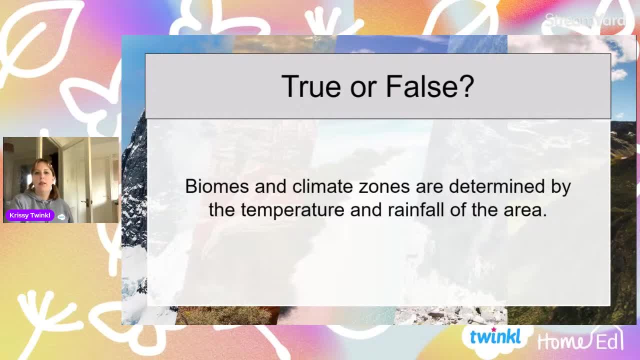 by the temperature and rainfall of the area. So do we determine biomes and climate zones by temperature and rainfall? Yes, A biome is to do with the animals, the plants, the physical geography, the physical things that you can see, and its climate. 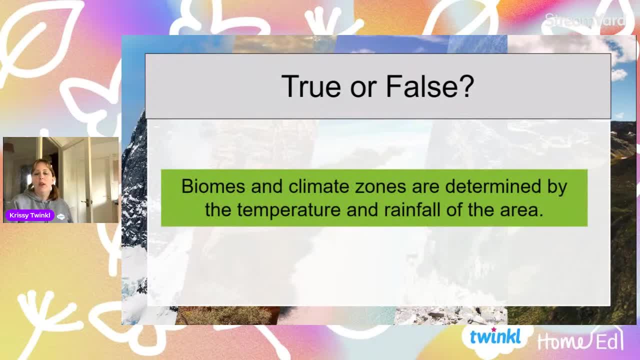 Absolutely This is true. So a climate zone is definitely determined by its temperature and rainfall. OK, that's, that's exactly what a climate zone is. But the biome will also be determined by temperature and rainfall, alongside other things. So it will be. 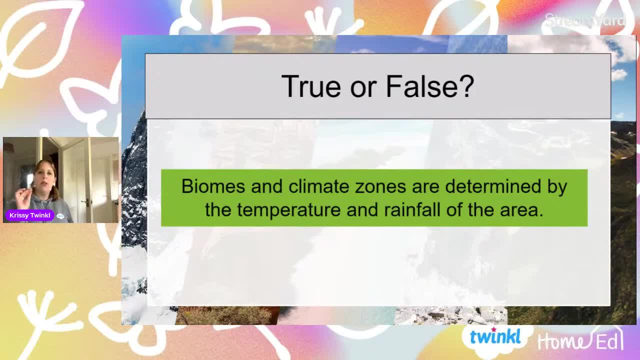 determined according to animals, vegetation, physical geography and climate. That's absolutely true. This is where it's getting tricky. A climate influences biomes, but biomes do not influence the climate. You think that's true? What do you think that's false? 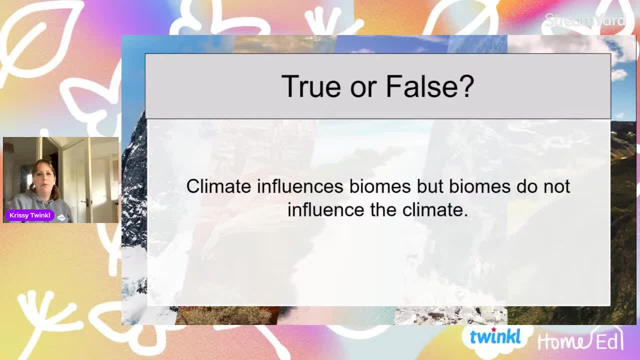 So climate influences biomes, But biomes do not influence the climate. What do you think? Bit of a kind of mixed bag there. It's true, So climate does influence the biome, but the biome doesn't influence the climate. So it doesn't really. 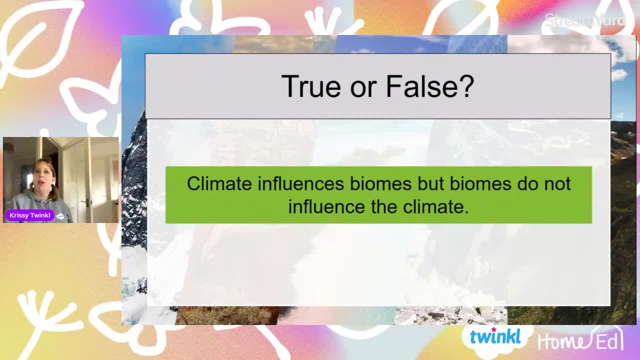 If you think about a rainforest, the fact that it's got how the monkeys swing around in it and the fact that it's got certain vegetation in it, so it's got particular palm trees or mahogany trees in the rainforest, that doesn't affect the weather that you 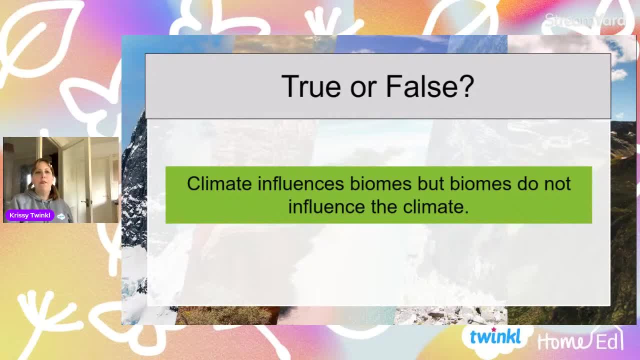 would find, does it? Can you see that? So the fact that I've got rabbits hopping around the field behind me and I've got an oak tree and I've got a sycamore tree in my garden, And that's all to do with my biome, because we live in a deciduous forest- 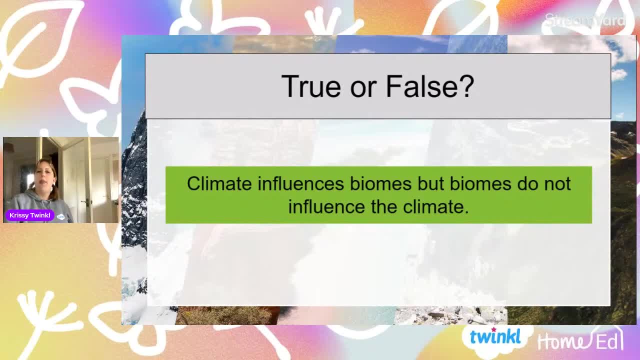 But the fact I've got all those things, that's not going to affect the weather, is it? And it's not going to affect the climate, is it? So that's a really important one. What a biome is is is partly influenced by its climate, its animals, its vegetation. 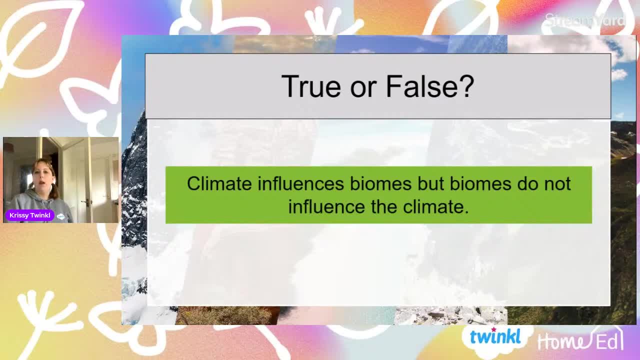 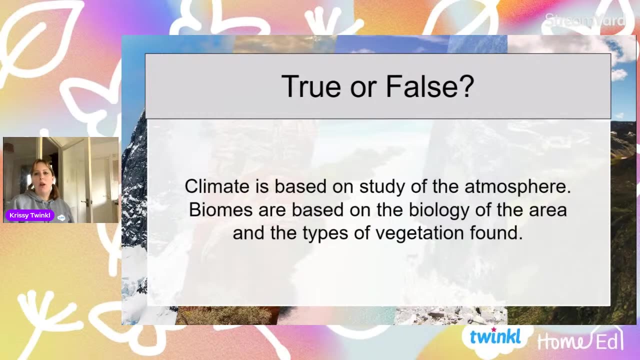 But a biome doesn't- doesn't influence climate. That's to do with something completely different. Does that make sense? We're going to look at what influences the climate next week. So climate is based on a study of the atmosphere. Biomes are based on the biology of the area and the types of vegetation found. 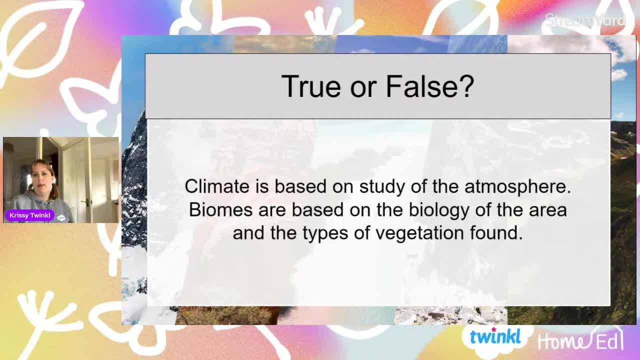 Is that true or is that false? So climate is based on the study of the atmosphere. Biomes are based on the biology of the area and the types of the vegetation found. Is that true? It absolutely is true, And that is the point. 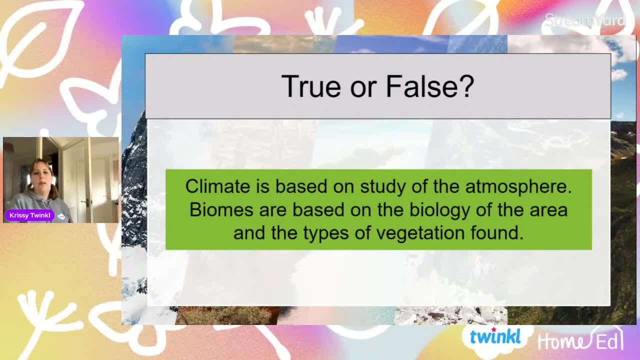 There's a fundamental difference. A climate is based on the study of the atmosphere. Don't matter what trees there are there, It don't matter what animals you've got there, Doesn't matter what the physical geography is. A climate is is a is is figures of atmospheric study. 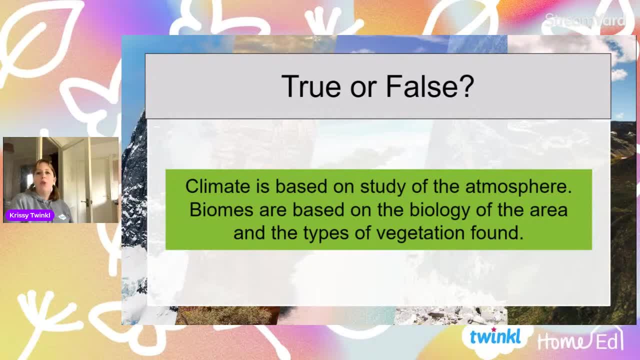 So that's exactly what climate is. But biomes are based on so much more: The biology, the type of vegetation, the animals, physical geography. So that's, that is the clear difference. Climate is purely The study of the atmosphere. 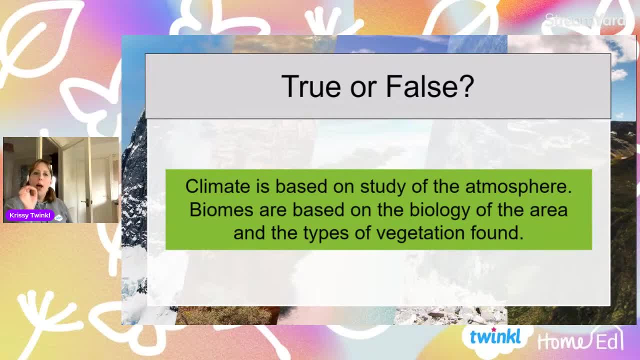 It doesn't matter what vegetation or animals there are, But biomes the reason that vegetation may grow in that area. So I could try and grow a banana tree in my garden, but it won't grow because I've got the wrong climate. so biomes are influenced by climate. 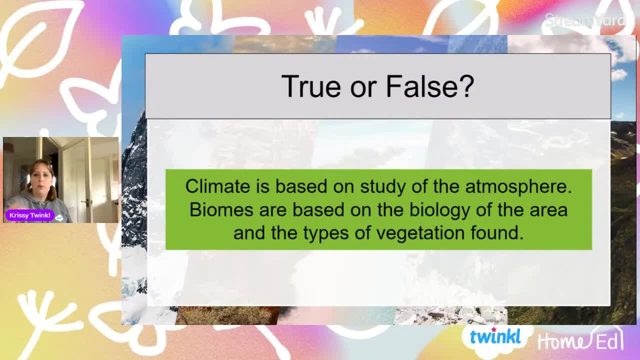 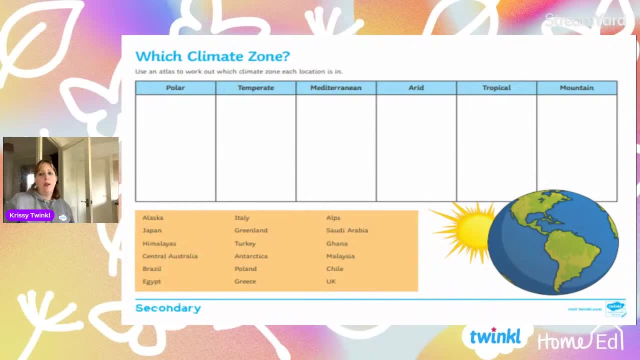 but also the biology, the vegetation, the animals. Is climate change caused by humans or the natural world? Depends on what scientists you talk to. So some scientists will say that we have had climate change. Think about the Ice Age. We've had climate change since Earth began, and quite extreme climate changes. 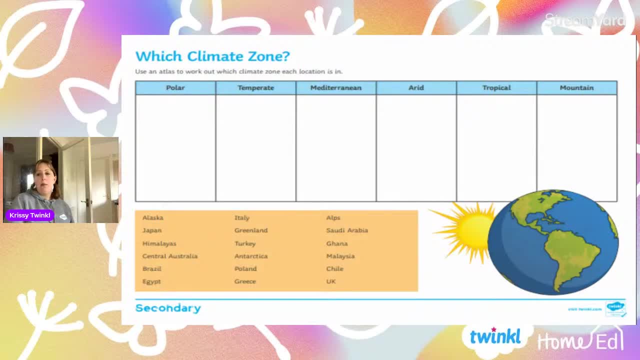 And so a lot of scientists will say that climate change is a natural process caused by the natural world. But most scientists will argue that the climate change we're experiencing now, which is the Earth heating up, is being sped up by human behaviour. I hope that answers your question. 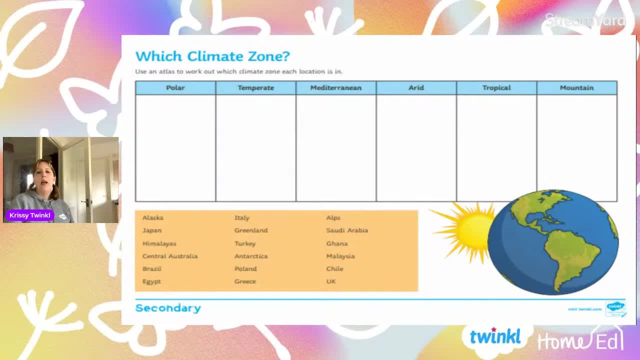 So yeah, so that's a big rundown on climate zones and a big rundown on what the difference is between climate zones and bios. If that bit was a bit too, then please don't worry. It's just a little thing that I think is. 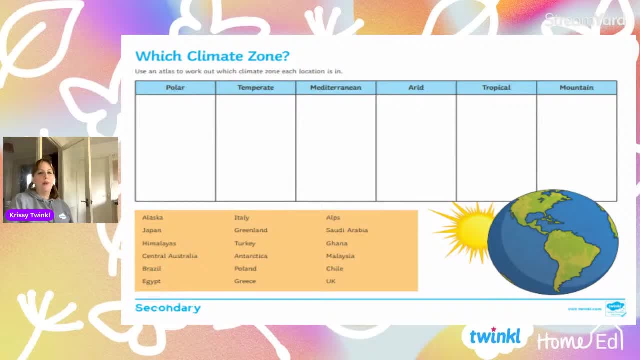 really important because some people who aren't top geographers, like you guys, interchange biomes and climate zones and that's why I wanted to cover it, And I could see that in the chat that some of you guys were doing that, And it's totally normal. 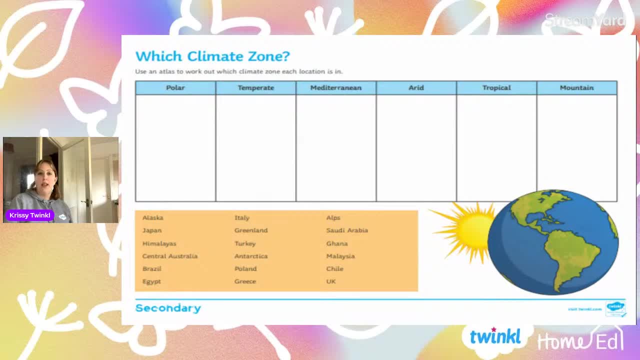 People, just people, just do it, unless you really deep down study geography like you guys are doing. People interchange climate zones and biomes And it's so important if you don't really understand the difference, It's just important to understand. they're definitely different. 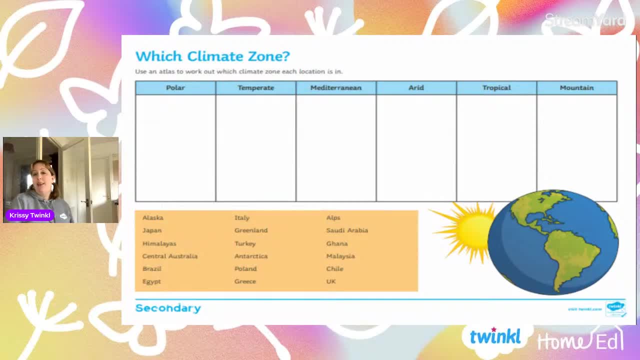 And if you go and look at a map, if you've got an atlas at home, go look, because you should have a map there on climate zones and there should be a map there on biomes and you can compare them. Get the two maps and look at them. 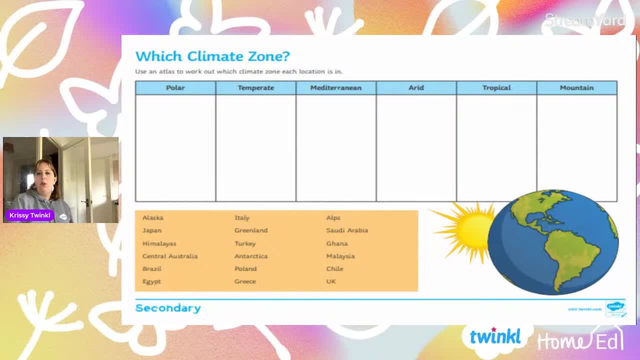 Or you can find maps of climate zones and maps of biomes over on Twinkl. Now up to you. But what I recommend you doing now is this lovely worksheet. I've linked it in the copy above or below, depending on what you are using. 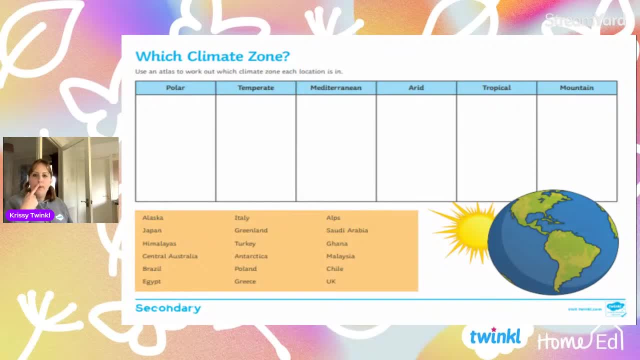 So you can click on it and it will download it out of the resources lesson pack. And this is about you doing a bit of an atlas study. If you put a globe, you can do it on a globe, But it's looking at these particular 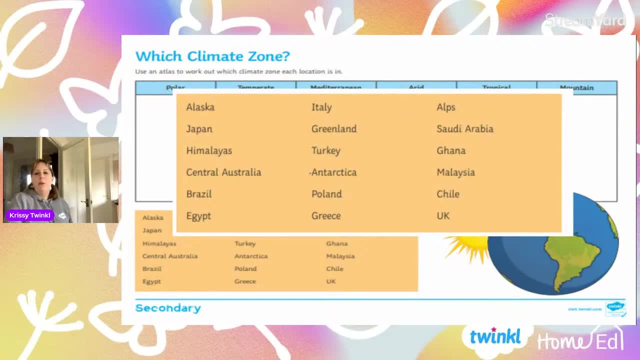 countries and finding out which climate zone they are. So you're going to need to get your climate graph, climate map. Getting the wrong words here. Look for Alaska. What climate zone is Alaska? Get your climate map. get your atlas. look at Greenland. 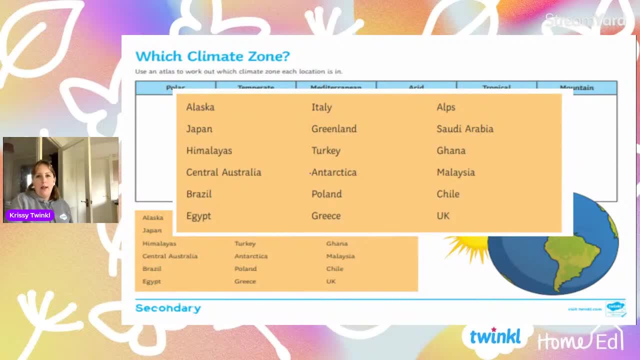 What climate zone is it? OK, does that make sense? So if you want, do a little bit of an atlas study, I love a bit of an atlas investigation. If you don't have one, you can download a map, world map and a climate map from Twinkl. 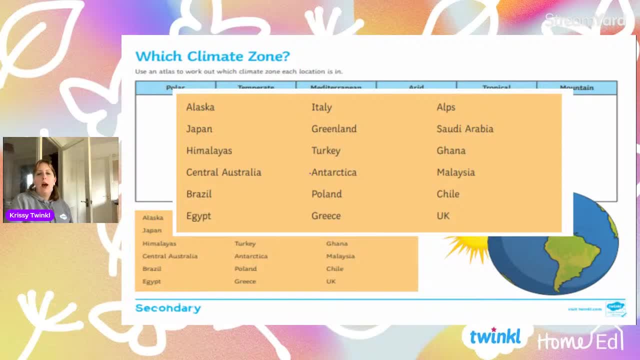 But definitely have a go at this and look all around at all the different climate zones and also add some of your own countries in, if you would like. Another thing you could do, which is in the resources pack above, is you can colour in your own map of climate. 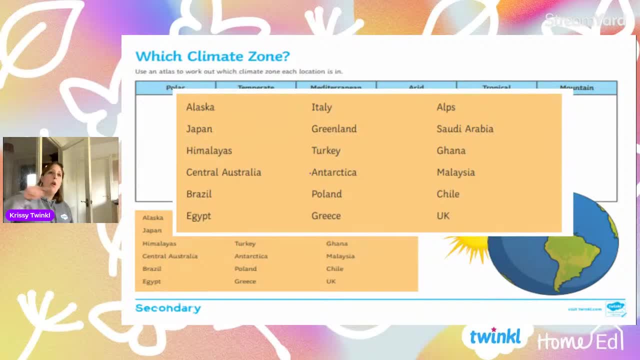 zones and you can label all the different climate zones and you can write around the map about all the different climate zones. If you really want to go to town, that activity is there too. So thank you so much for joining me And I will see you next week. 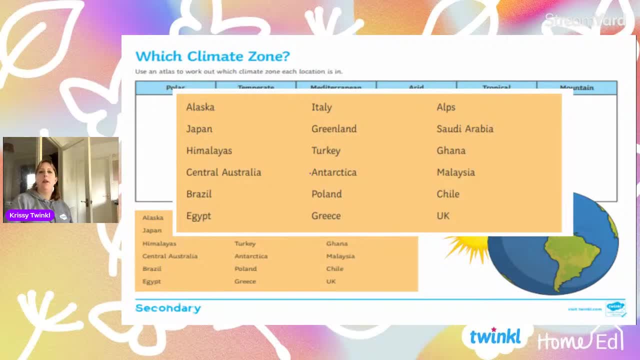 Where are we going to be looking at? Why do we have different climate zones? So, if it's not to do with the vegetation and it's not to do with the animals and it's not to do with the physical geography I can touch, why do we have a temperate climate zone? 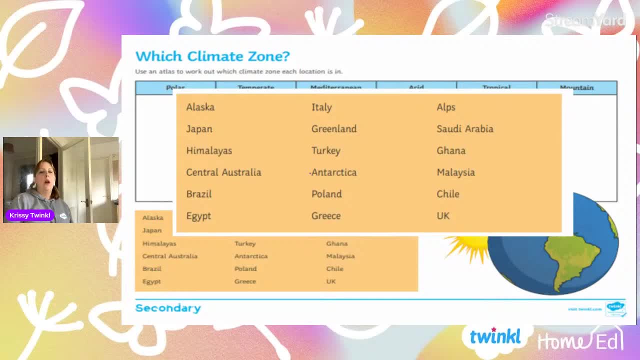 Why, if I go to a tropical climate, why does it have a tropical climate, and so on. So that's what we're going to look at. OK, so I will see you next week. Bye, bye.